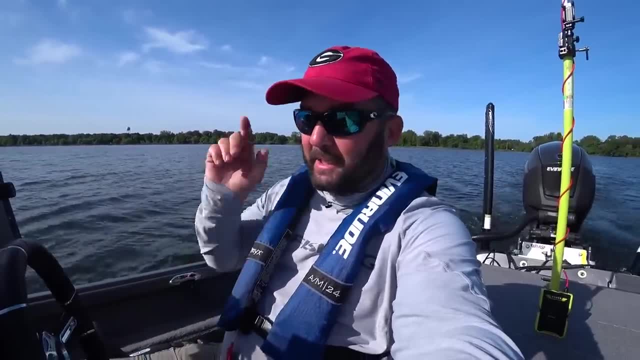 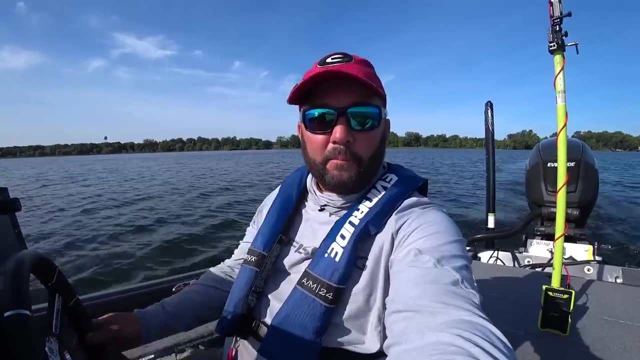 one. I am not a boat expert. What I'm good at is getting a boat on the water and getting back safely, and that's what we're going to talk about today. So don't hold any of these crazy little details like pitch of the prop and all that other stuff over my head, because I don't understand them. 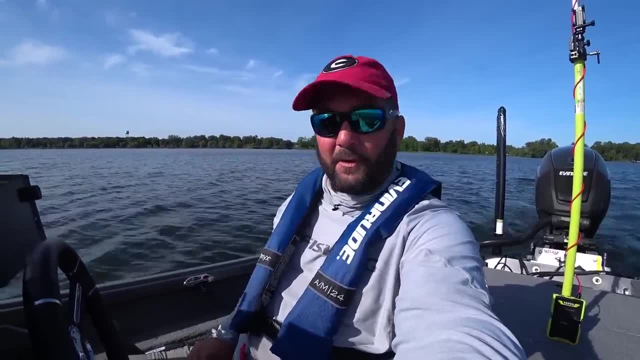 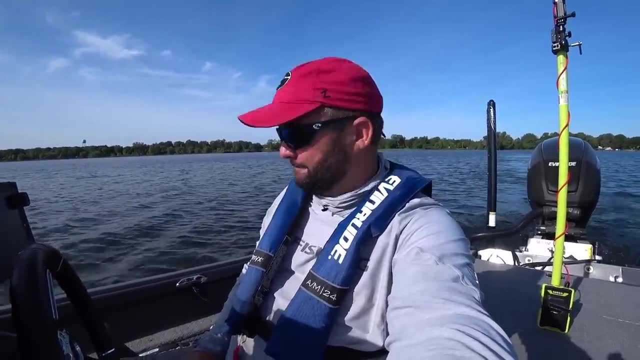 and I could care less. I let the engineers take care of that. So let's get into boat operation: How to get out on the water, how to operate a boat safely and how to get back safely. All right, so to start with, 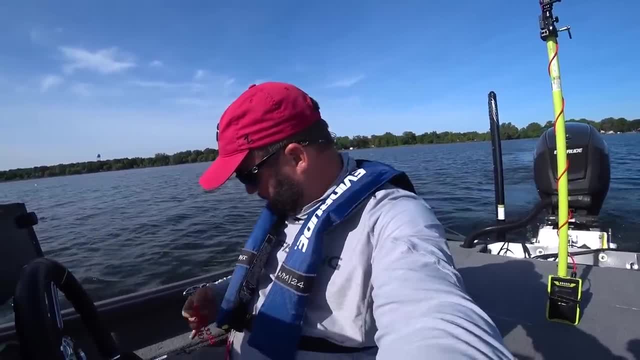 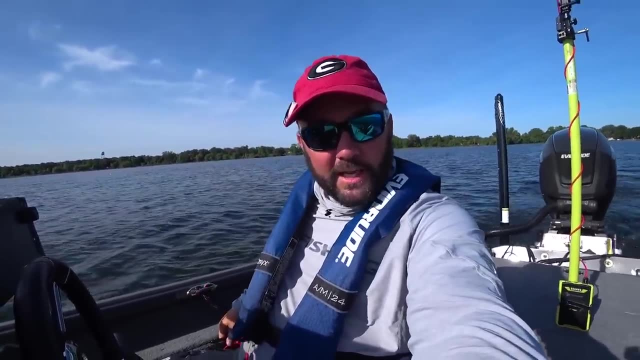 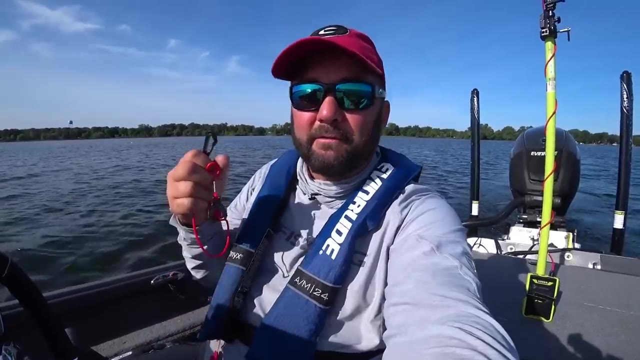 always wear your PFD And this little sucker right here. this is the pull cord to your kill switch. When you get knocked out of the boat, your engine shuts off and your boat stops and it doesn't go away from you. And if, for any chance, you didn't get knocked out or you come to, you can get back in your boat. 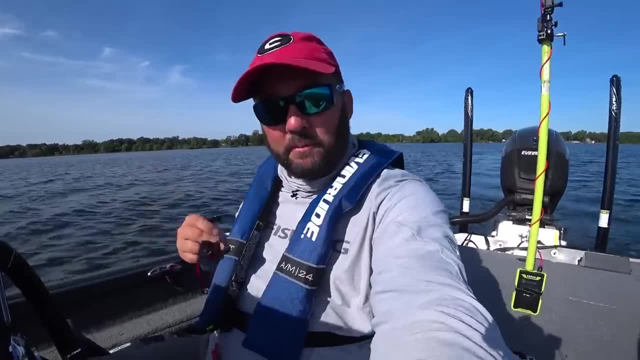 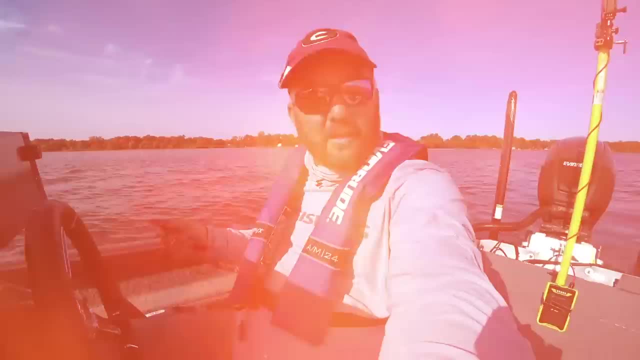 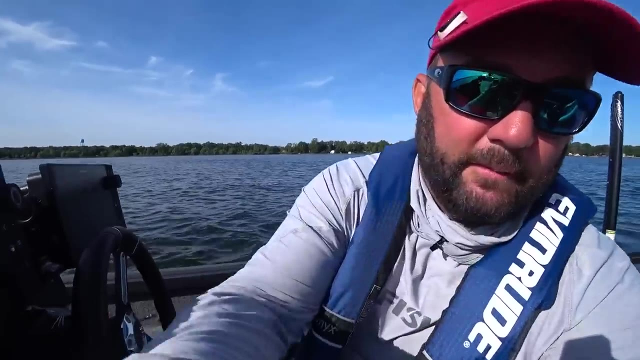 because your boat will be right there. So always hook your kill, switch up to your PFD and always wear your PFD when that big motor is on. Safety, And that's what it's all about. All right, so let's go over some parts and pieces of the boat. So, to start with, let me pop this camera off the tripod. 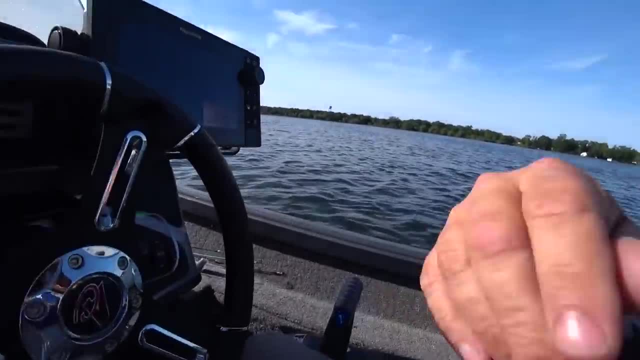 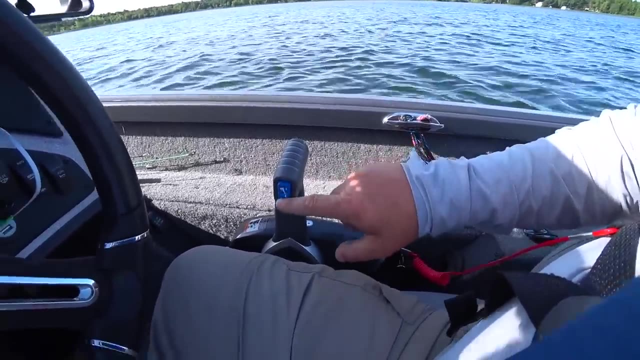 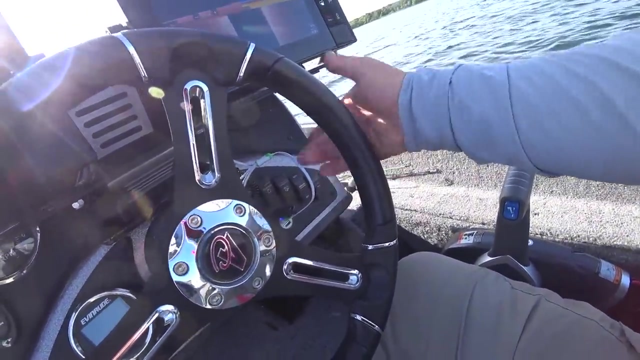 All right, All right. So first of all, here's your throttle This right here. this is your trim switch. This is very important. You use this a lot. Some boats have the trim switch in a little almost like a turn signal, whatever, a little toggle right here or right there. So one thing to understand is that 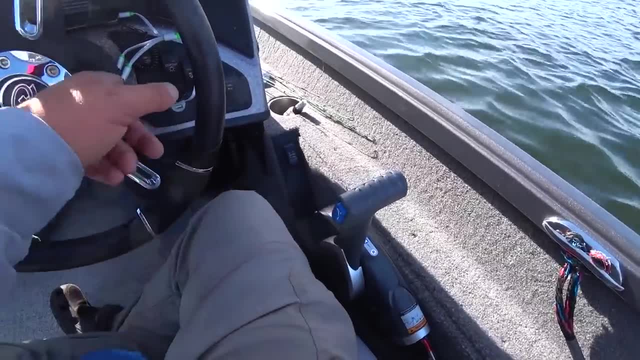 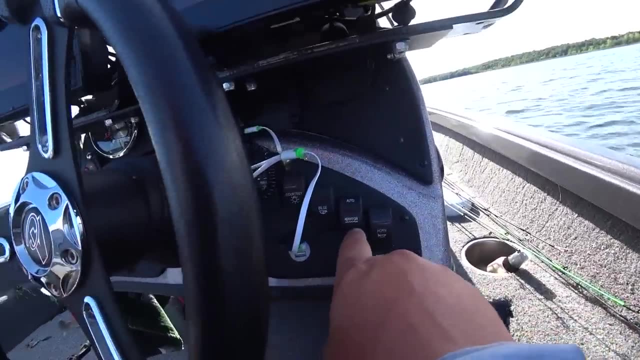 every boat is a little bit different, but I like mine on the handle and I hope to get one on here one day, but it's. I just find it easier to use it on the handle. You got your horn, you got your aerator, your pump for your, for your live, well Builds pump, which as many 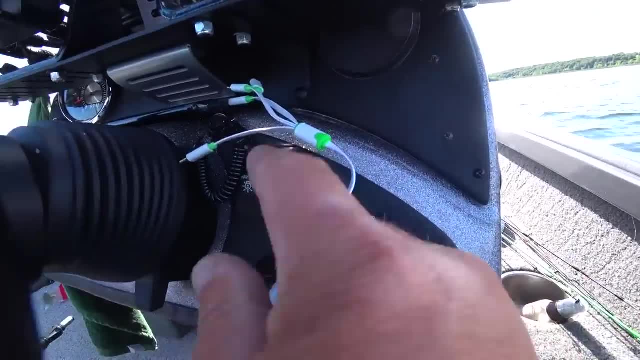 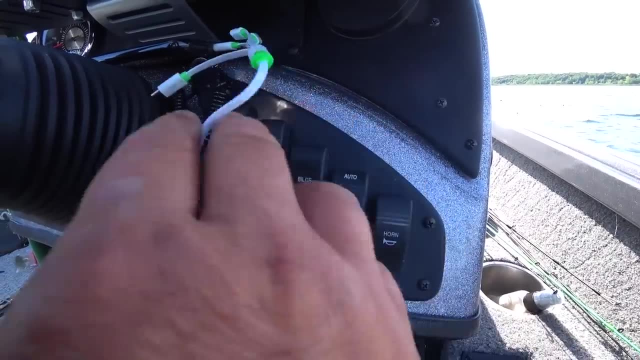 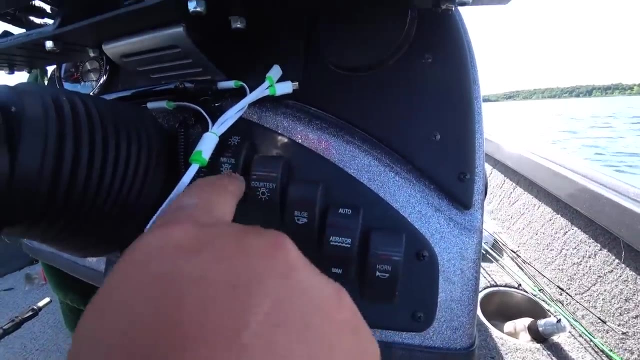 times as I've had leaks in boats, I I habitually will test it throughout the day, just making sure that the the the builds doesn't have a whole bunch of water in it. Courtesy lights, which is just a light that turns on here in the cockpit, And then your nav lights, And when it gets after. 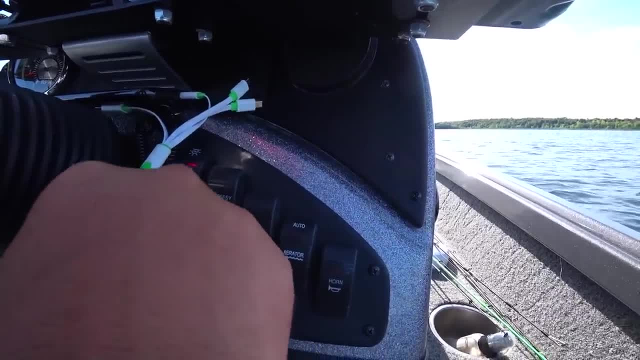 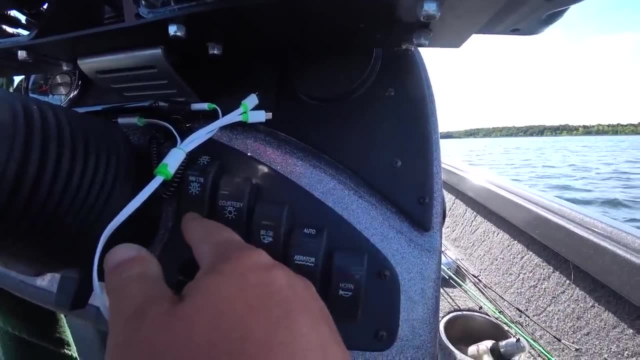 this: when the sun goes down, you put your lights out And you turn your nav lights on. So you've got the green and red light up front and you've got the light on the back of the boat. always, when the sun is not up, have those in. have that turned on? 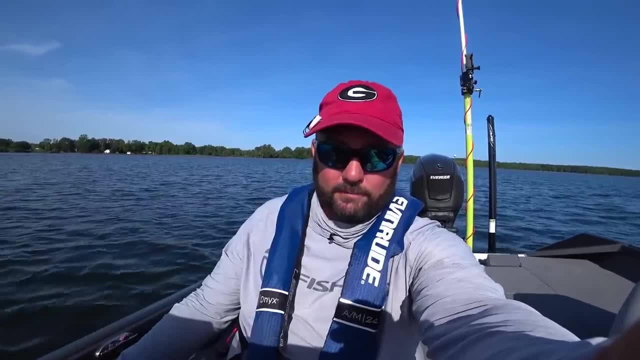 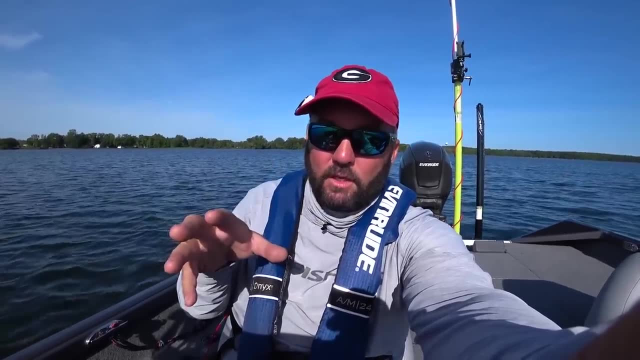 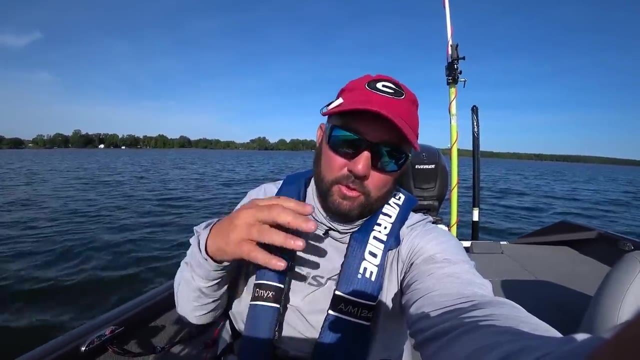 All right. So once you have the boat in the water, okay, And I'm going to- I'll put a link right here to the to how to launch a boat by yourself, which most, most states will let you power launch it like that, like I do in that video. but check your state regulations and check the regulations at the boat ramp and make sure that you can power launch it. 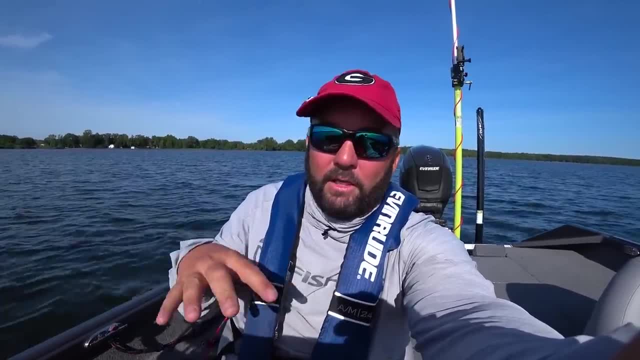 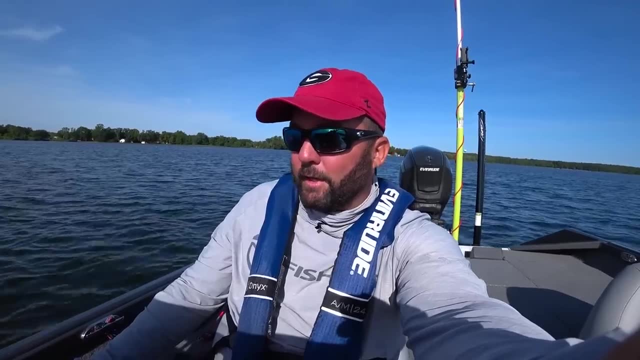 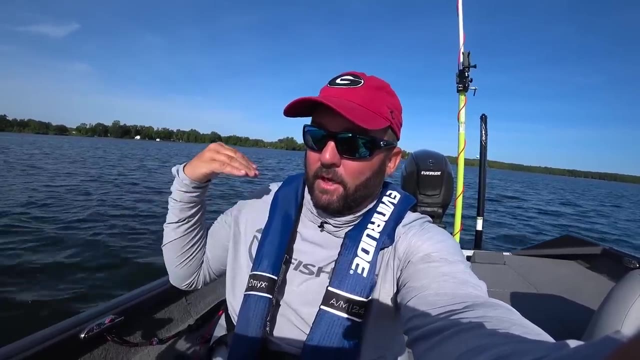 If not, there's a different technique. But I have rarely come into into contact with a boat ramp that wouldn't let me at least idle off the trailer, But anyway. so you put the boat in the water, you get it out away from the the boat ramp, you get it past the no weight buoys and then you're ready to take off. 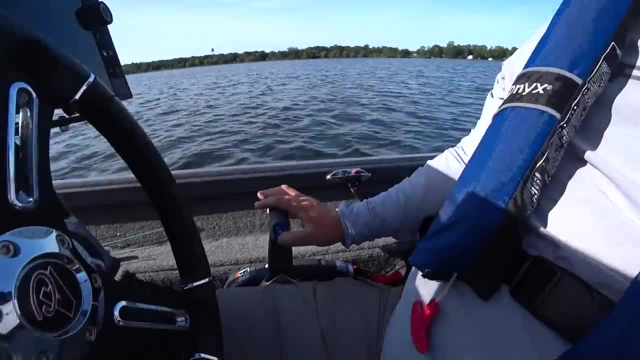 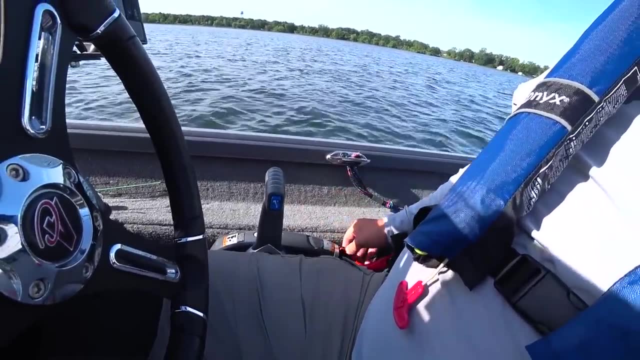 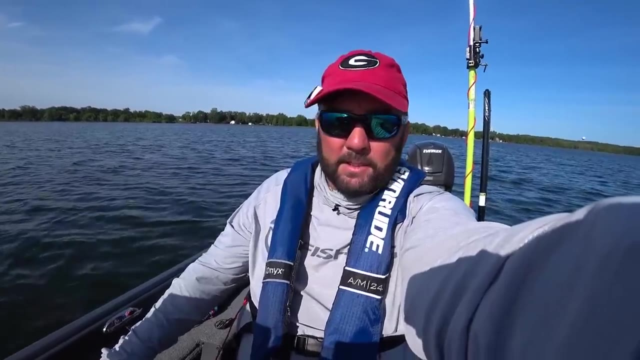 You're ready to get it up on plane. So what you do is you take and you run that, hit that trim switch all the way down. Okay, All right. So your trim is all the way down. Take this sucker up. And I'm going to explain this before I do it. 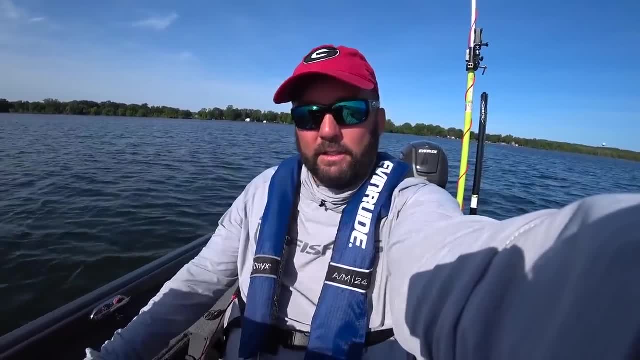 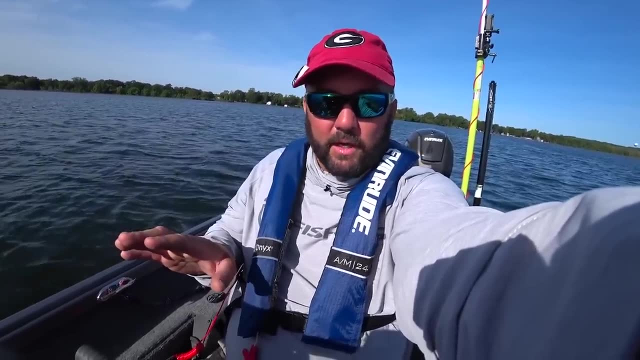 You push the throttle all the way forward, or most of the way forward, get it up on plane, And I back off a little bit, because I hardly ever run my boat at full speed, but you can run at full speed And if you want to run it and see how fast it'll possibly go, what you do is you go ahead and floor your your uh. 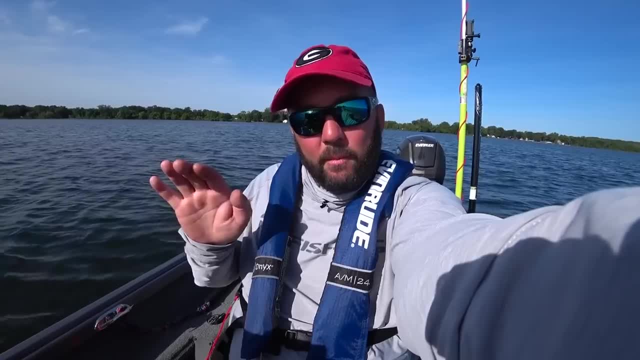 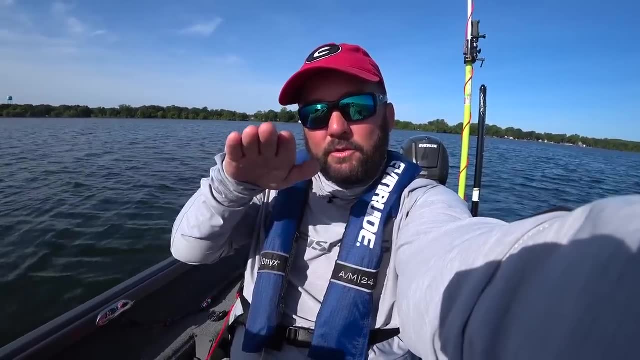 your throttle all the way down and then hit that trim up And that trim will lift the front of the boat And then you lift it up until your boat starts to to purpose just a little bit and you'll feel it just barely starting to start hopping. 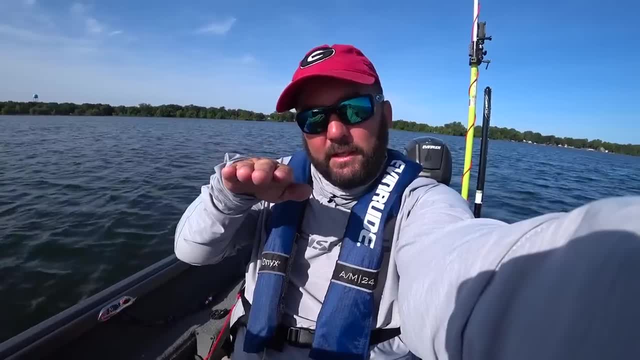 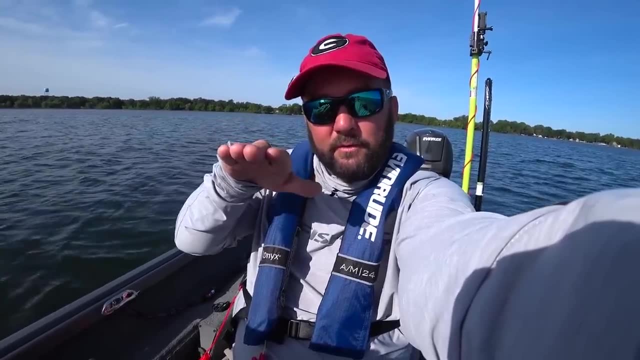 If you're not going over top of any waves, trim down just a little bit and it'll stay up on planing To give you your top speed. Um, what I typically do is I will get it up on plane, I'll come off the throttle a bit just to save gas and I don't need to get anywhere fast. 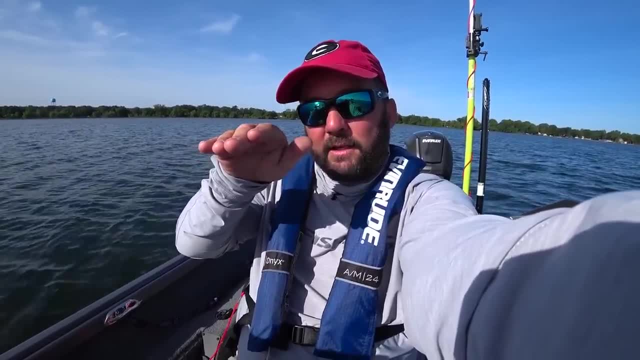 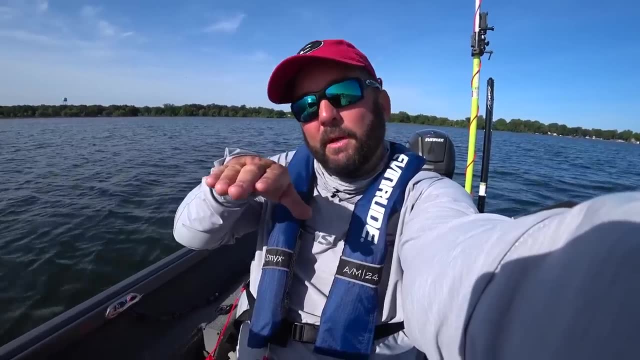 And then I will- Okay, will just cruise and I'll hit that trim up just a little bit again until it starts to porpoise, and then I'll come back down Slower speeds. it porpoises earlier, with less trim, Faster speeds. 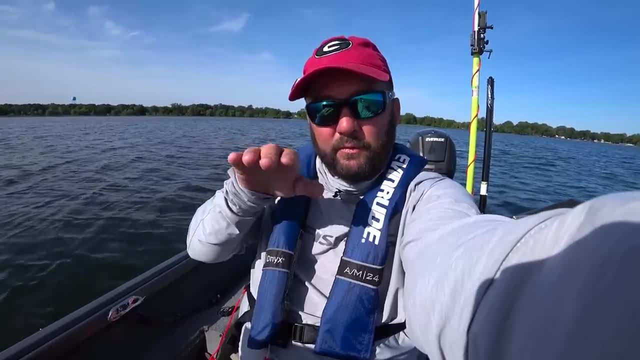 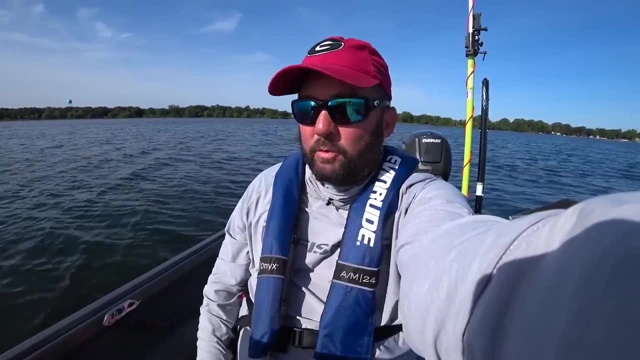 you can trim it up a little bit more and a little bit more, and it's just a matter of feel and playing out with your boat. I remember years ago I was captaining a high school- no, not a high school, It was a junior bass master's back in the day- and me and Ryan were sitting there on the. 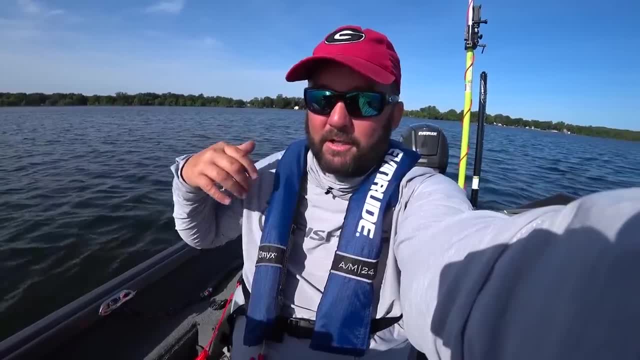 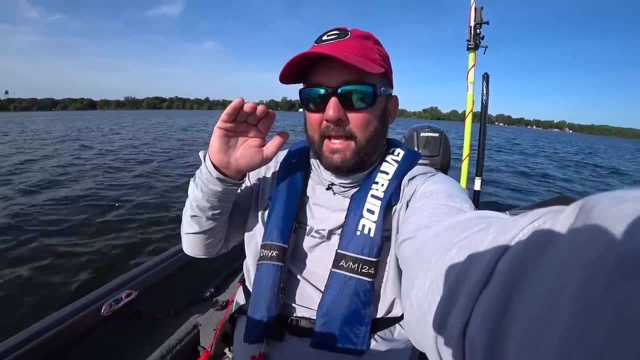 point. Ryan was fishing and I watched a brand new bass boat across the lake get put in the water. I know the only reason I know it was a brand new bass boat is this dude had never been in a boat and it was a nice sparkly red boat and he got it. He would hit the throttle, It would get up. 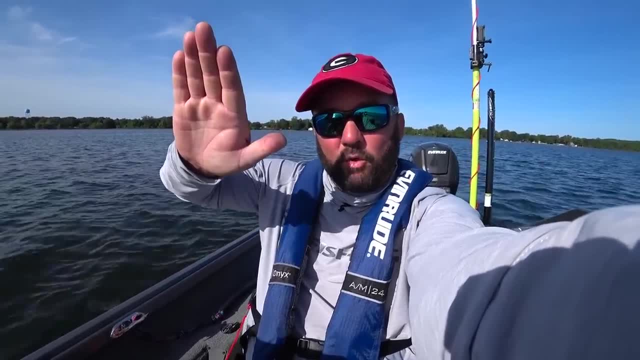 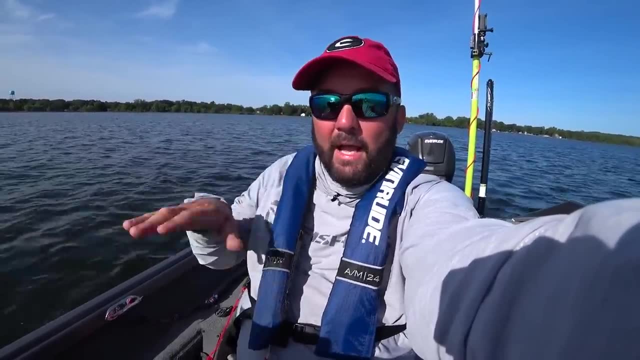 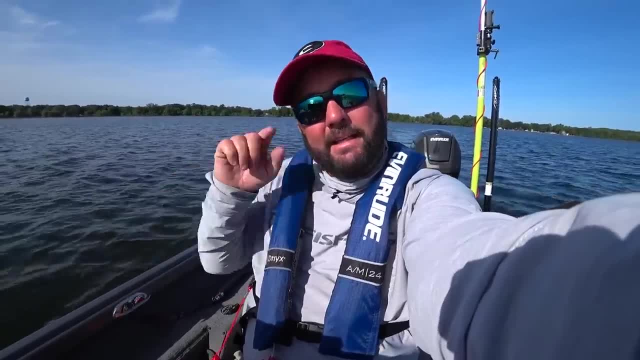 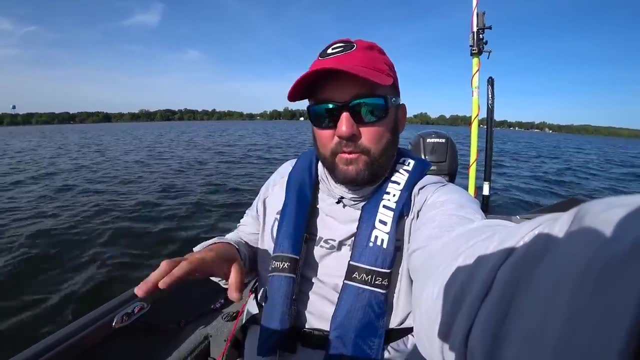 watched him idle back into the marina, put it on the trailer and take off. He never was told a thing about the trim. The trim is everything. Also, when you get into shallow water- less than three foot of water- I trim that motor up. I have a hydraulic jack plate. that's a whole different. 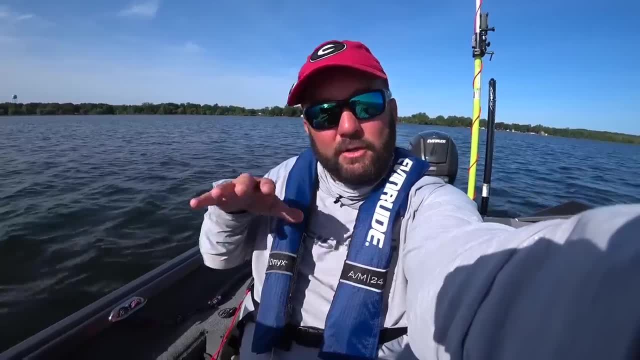 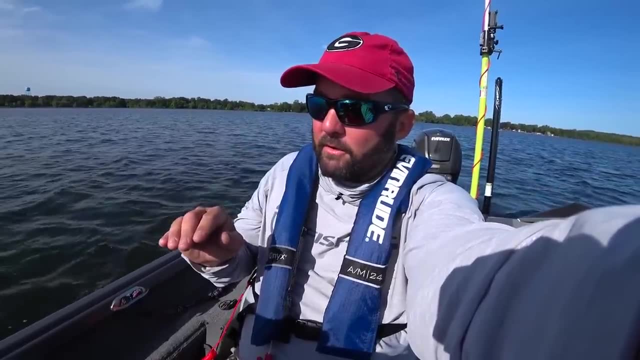 world. but I trim that motor up just so I don't hit anything, and I always make sure that I pay attention to my map and know when I'm in shallow water. I don't run high speed in shallow water unless I know the lake well. 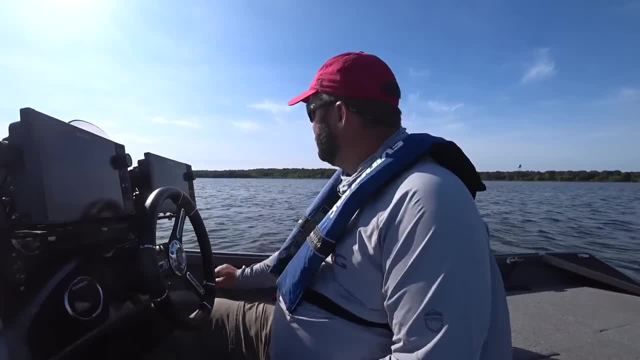 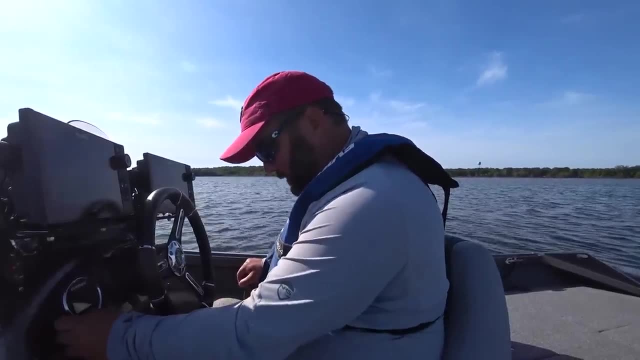 Yeah, dude, it's just about being safe. All right, so we're going to run through this. Now mine has a foot throttle, so actually let me switch to the hand throttle. That's what's nice about this new Evident route is you can switch to a hand throttle. All right, it's on. 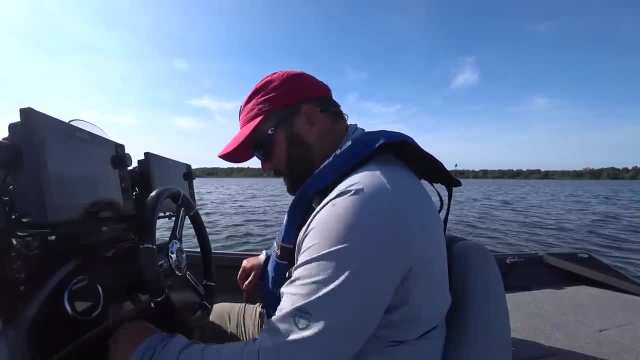 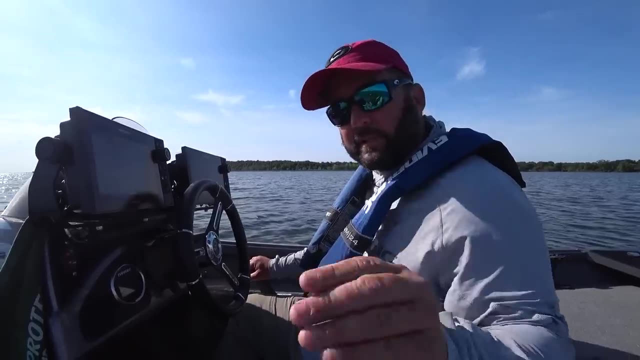 hand throttle, All right. so the first thing you do is you want to get it up on plane, and up on plane means it's up on the back half or back third of the boat and it's up on top of the water Here. 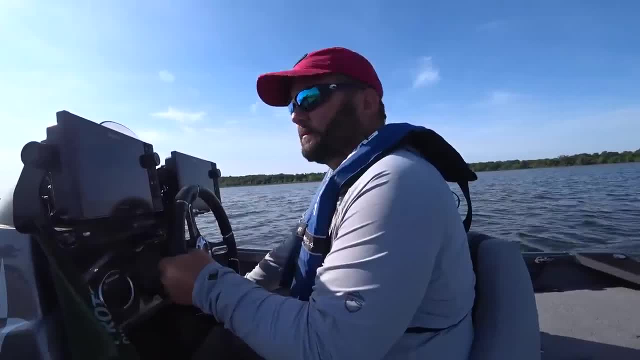 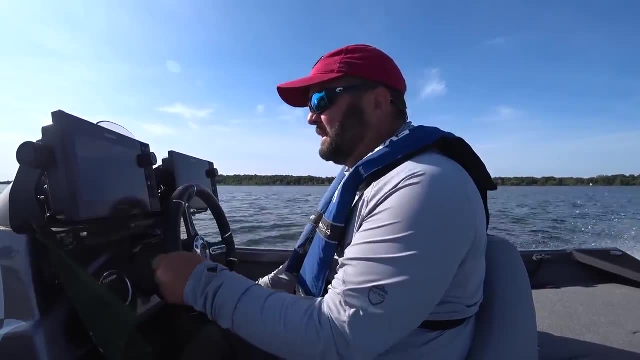 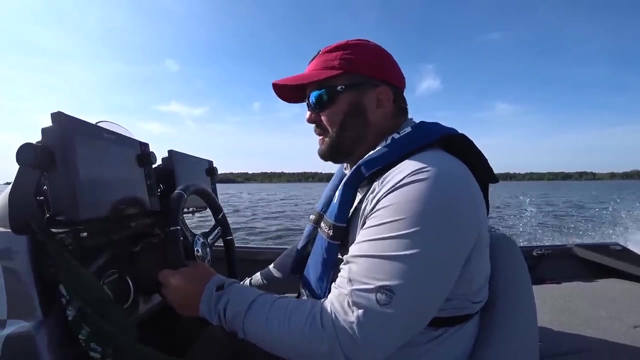 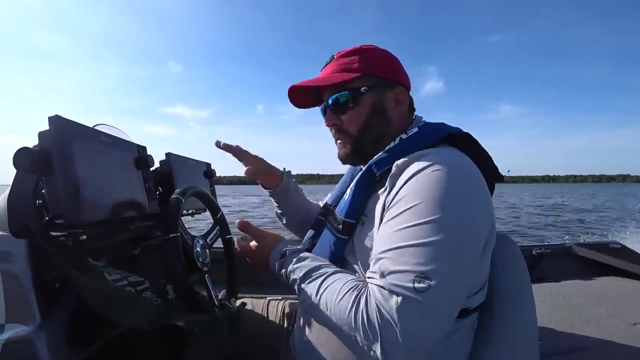 we go All right. so it's up on plane. I back off a little bit, get to a nice cruising speed and then I just start hitting that trim switch just a little bit and I haven't. I've started going faster, but my throttle, I haven't pushed my throttle down any. 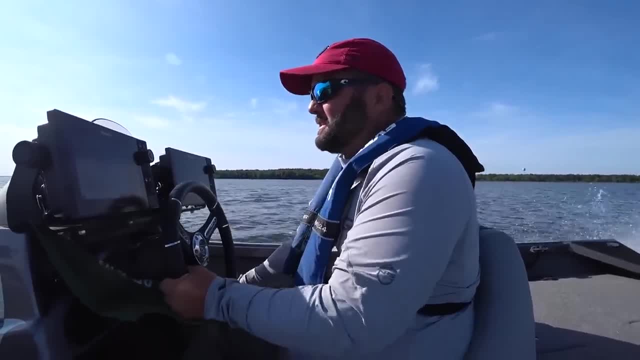 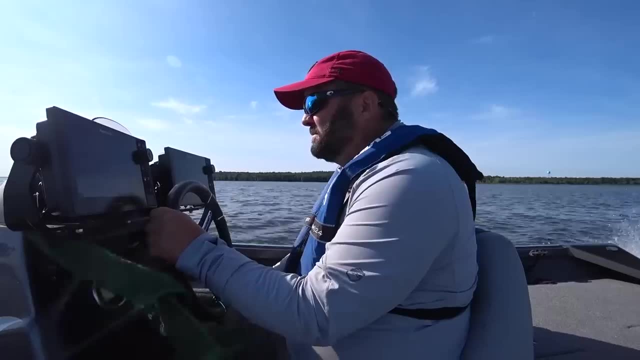 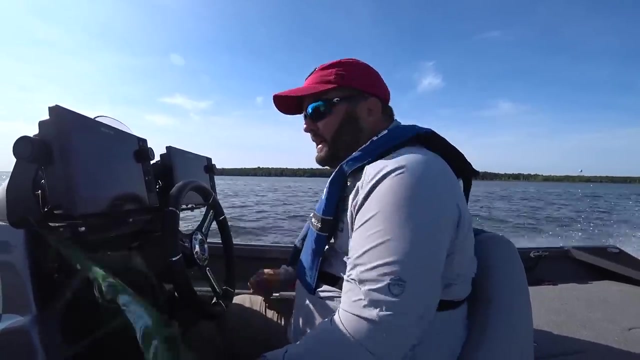 See, now it's starting to porpoise, so I want to keep my throttle up. That's what I'm doing, to come down just to hair until that porpoising stops. And that's how I do it. Now, if you want to go full speed, you just throttle all the way down. 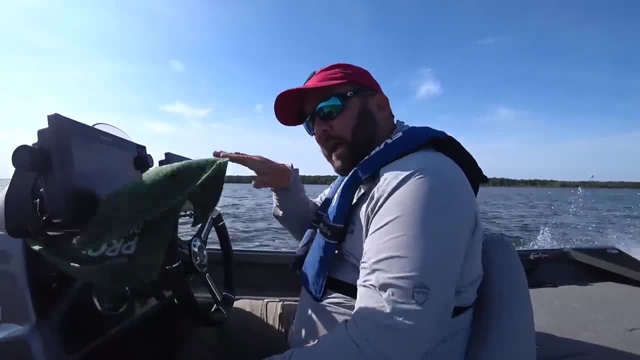 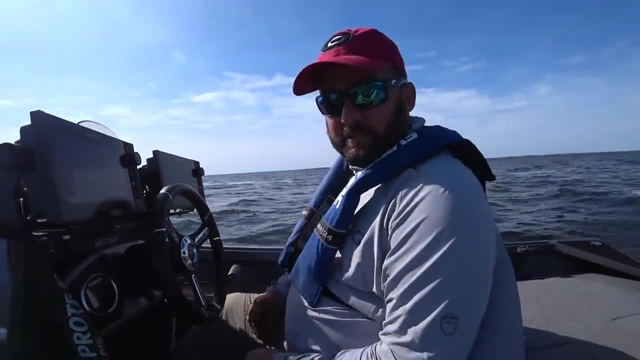 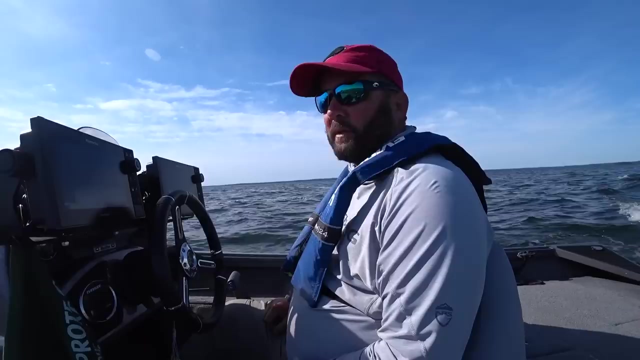 and trim it until it you get that optimum speed without porpoising. All right. so these are those rolling waves, Not a whole lot of white caps. Wind's not blowing- blowing really hard, It's like six, seven miles an hour, But because this is such a giant lake, I'm literally making a 10 mile run straight across. 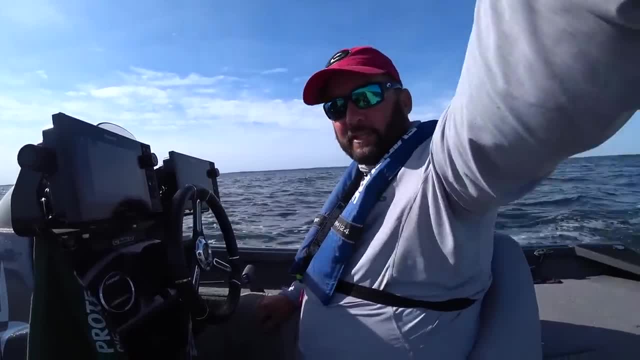 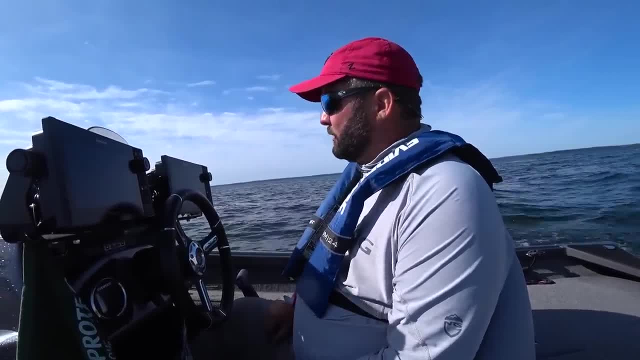 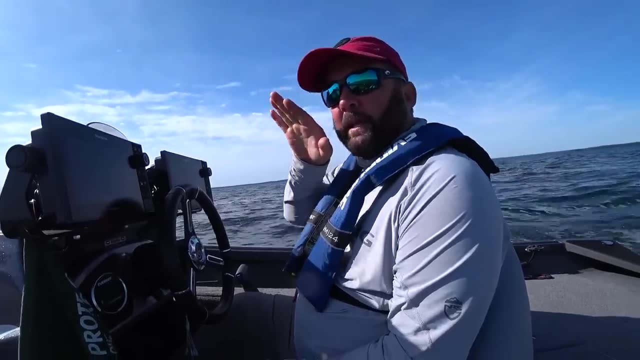 So I just want you to pay attention to how I'm feathering this throttle as I'm, as I'm riding over these rolling waves. Always, when you're coming down the wave, you want to let off, And then when you, you want to throttle up and come and let off when you're coming down the wave. 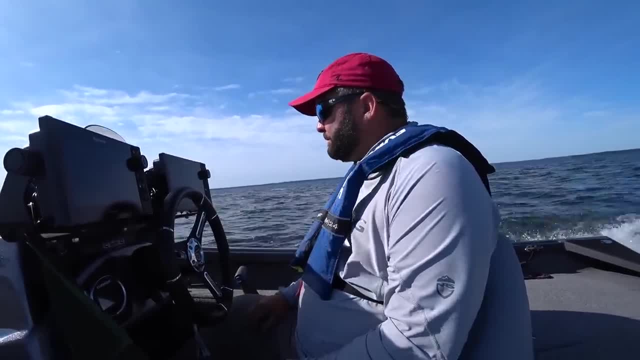 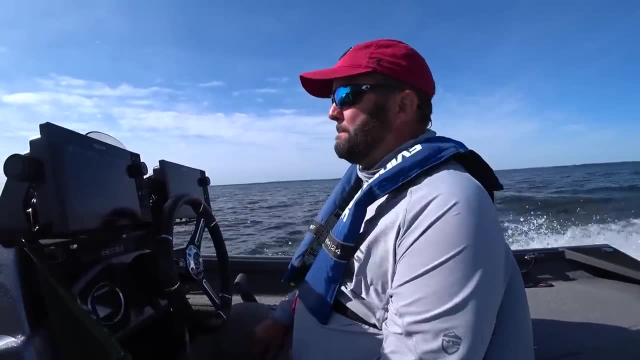 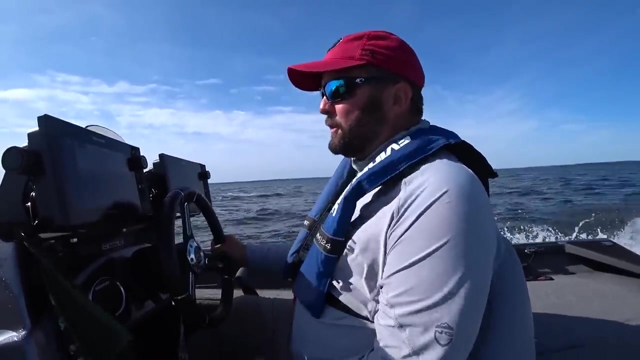 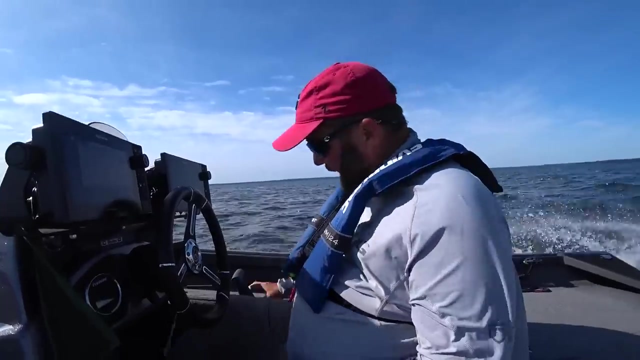 And I'm not in a hurry Now I've got my foot throttle. I'm using my foot throttle on this one, But it really doesn't matter either way. I'm using my hand throttle. I like to put my hand flat on here and just hold on. I don't know if you guys can see this. I'm holding my throttle. 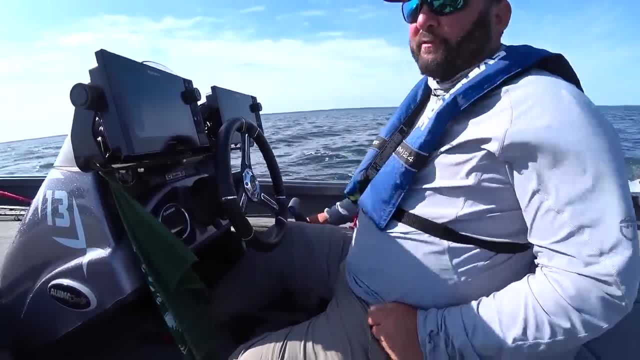 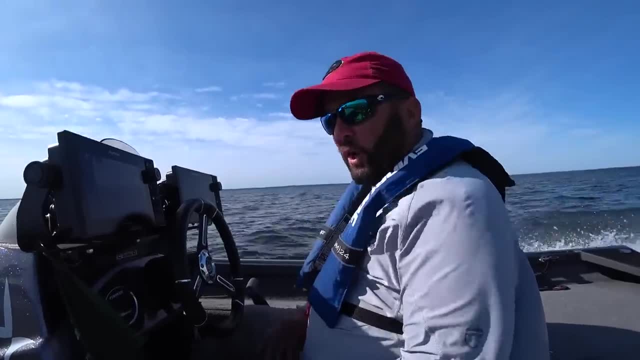 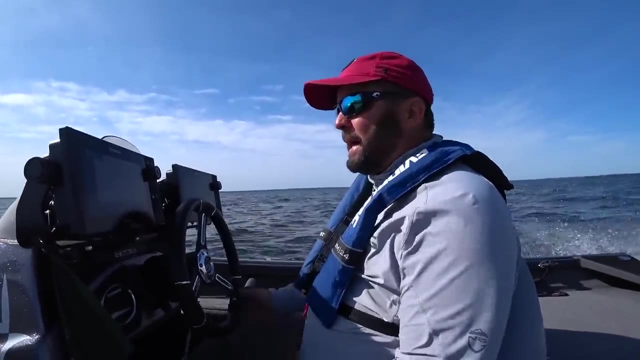 I'm holding my throttle right here and I'll feather it with my thumb. It just gives me more control over it. I can go faster. This boat can ride on top of these. It's just a little bumpy for me. I don't mind doing this, because I do need to make sure I'm going right in the right direction. 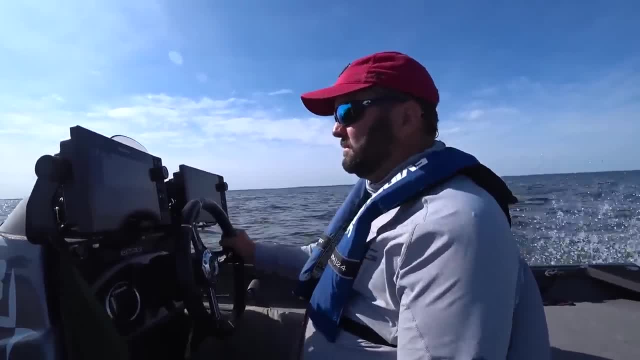 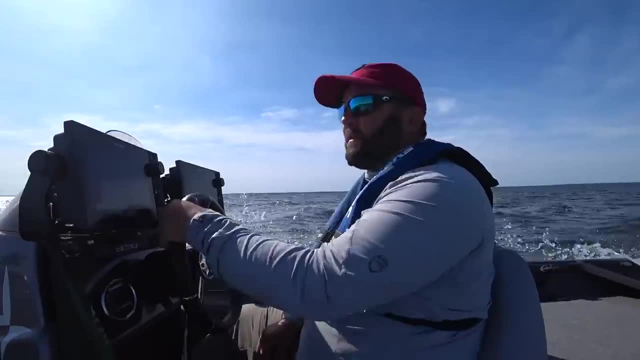 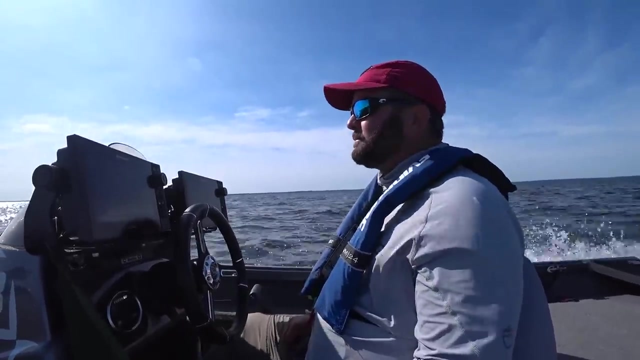 I'm just going to keep going. Every boat's different Deep V's are made for this kind of water. These flat bottoms not so much. You just got to know how to run them. This isn't a flat bottom. This is a modified V. 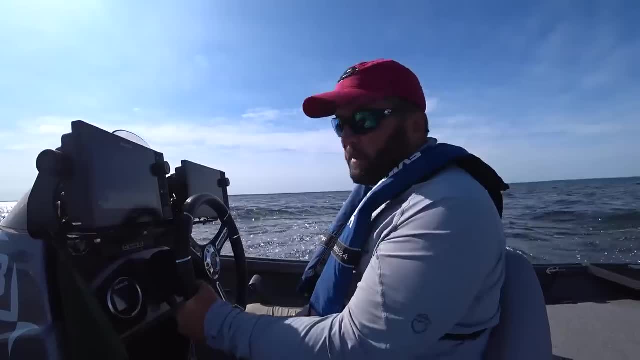 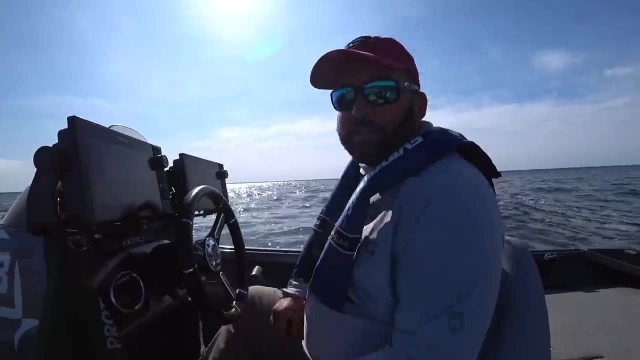 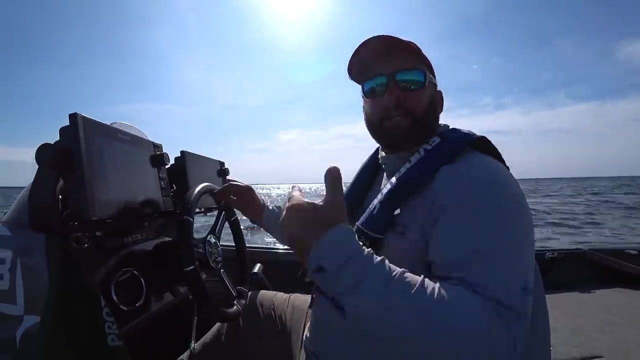 But anyway you get the picture. Every boat's different. Get to know your boat, Know what it can do. Alright, so all you guys who've watched Deadliest Catch, you hear about them running in the trough all the time And what it is is the waves are hitting you from the side. So you've got all these rollers and all these waves hitting us from the side. 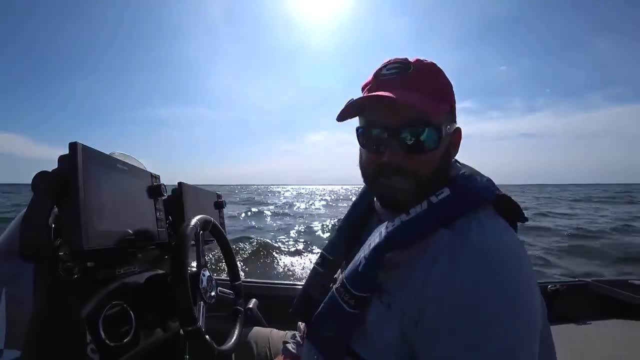 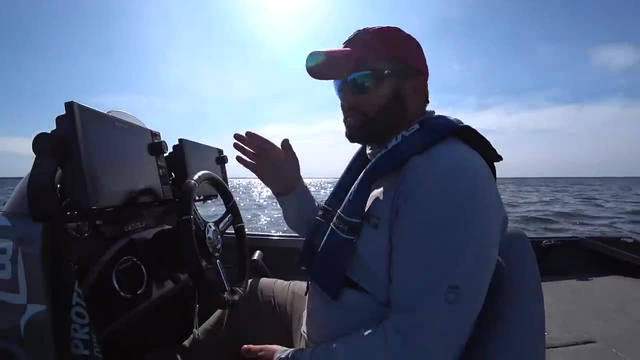 And really, when you're going slow like this, it can be really, really rocky. I mean, that's what they're doing when they're talking about fishing in the trough. They're going real slow and these big waves are hitting them from the side. 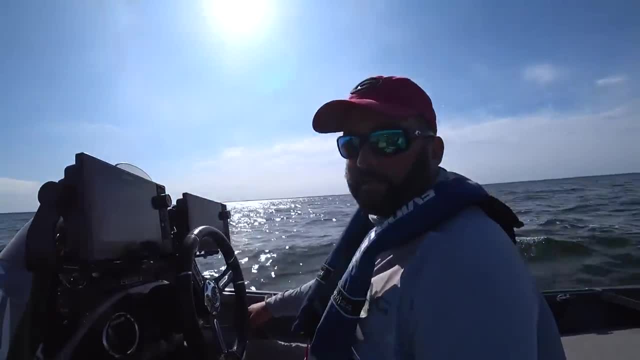 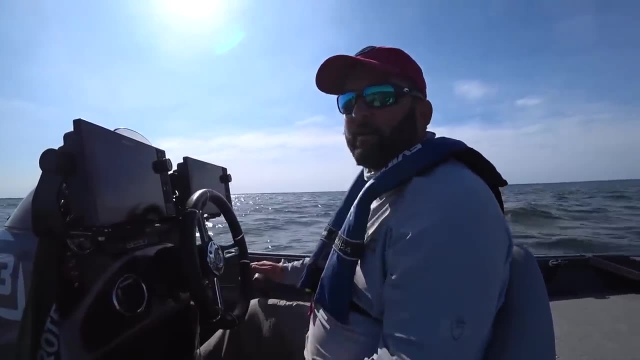 It's a smoother ride than when you're up on plane riding in the trough. You just have to be careful of the wave that's going to hit you at a 45 degree angle And that's just a matter of watching for it. It's not going to kill you, It's not going to hurt you, It's just going to get you wet. 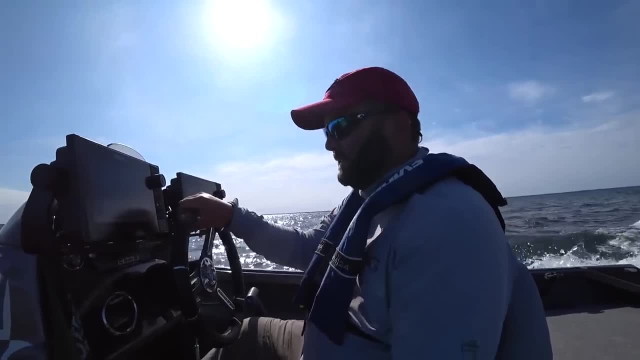 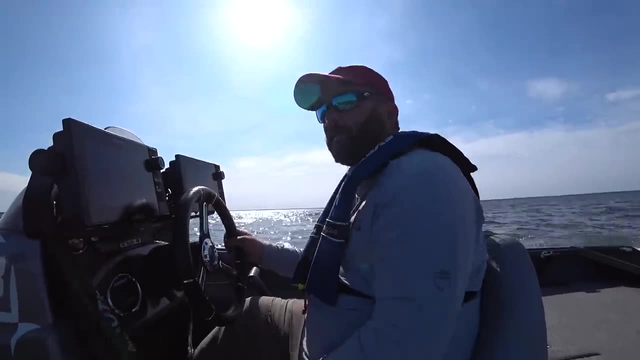 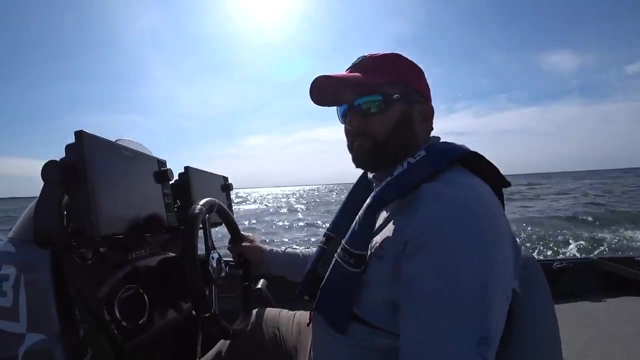 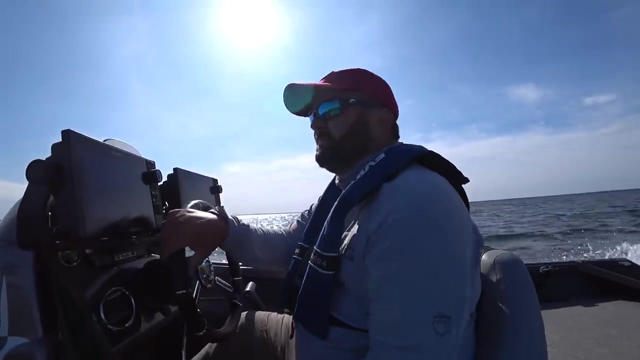 We're going to run in the trough for a second Get up on plane And I'm just keeping an eye out And I'm going fast, I'm trimmed off, I'm going down And I'm just riding the waves as I go over one. 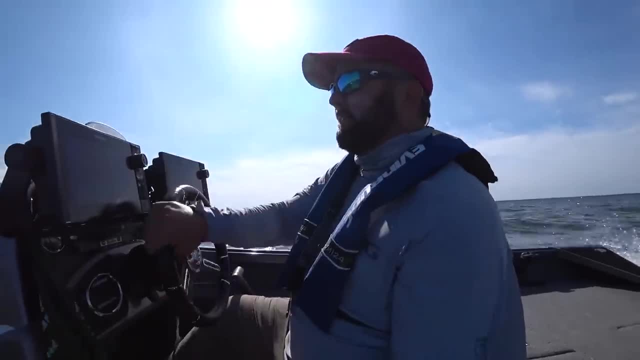 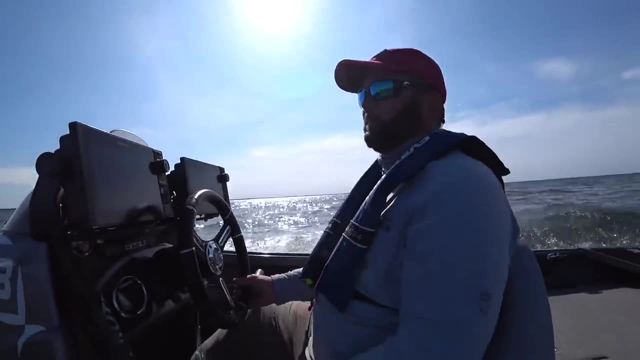 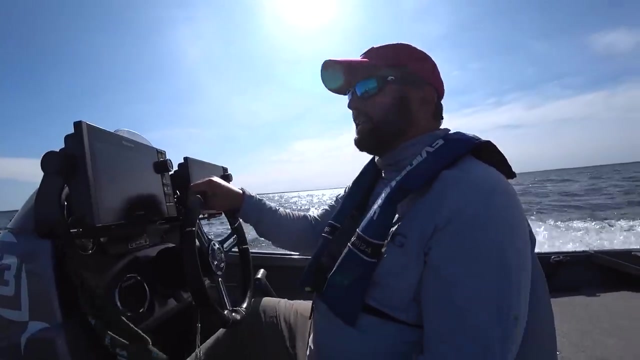 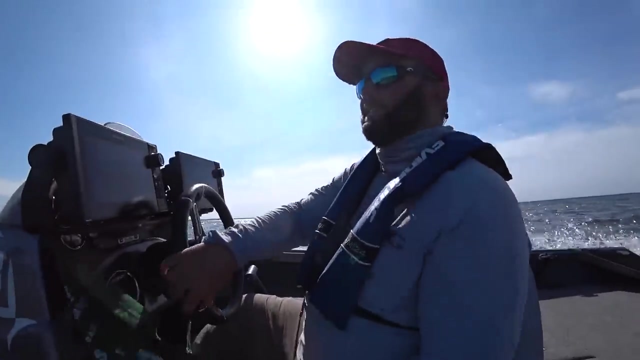 I turn into it a little bit. That's all it is. That's all it is. You've just got to kind of ride and steer with it And as you go over one you've got to turn it over. Not too bad. 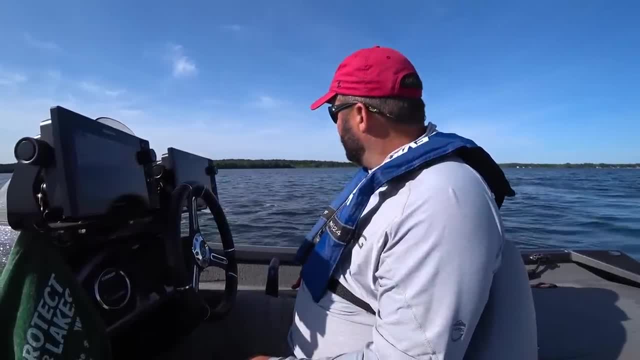 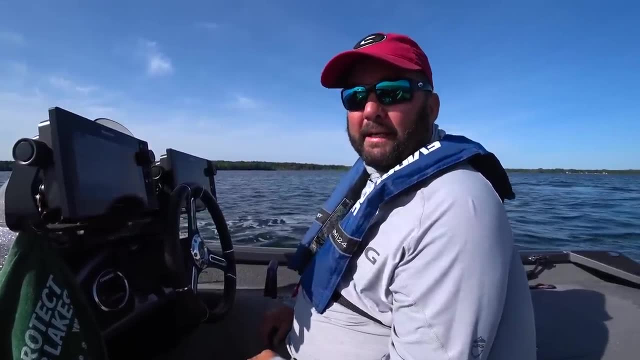 Alright, so let's get serious for a minute. When the weather gets rough on this lake- 10 miles an hour and it's rough, And it's a rough, tough ride back in, no matter what kind of a boat you're in. 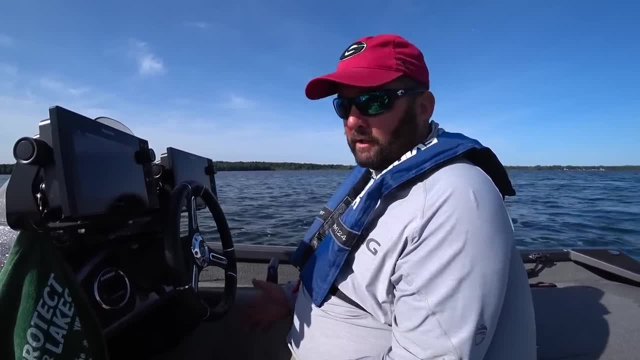 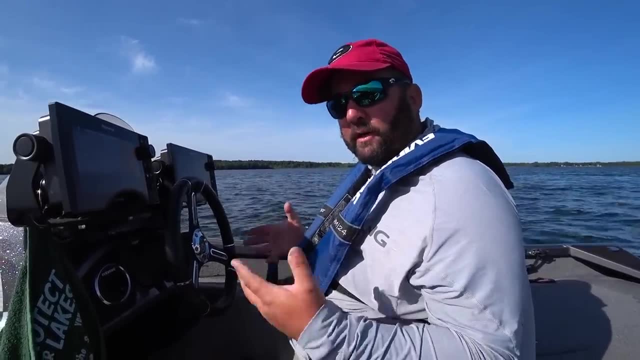 This aluminum boat. it's an 18 and a half foot aluminum boat. I love Alumacrafts because they are really really solid boats And they don't vibrate as much when you're in rough water, So you don't feel it up your back. 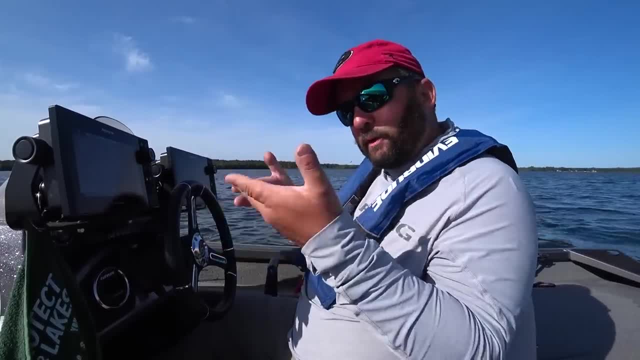 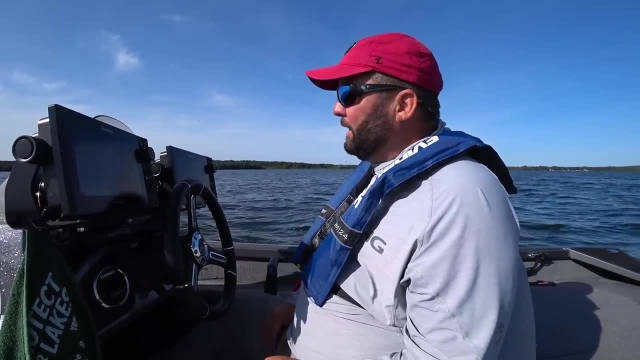 Other aluminum boats have welds right down the keel which allow a little bit of flex and vibration in the hull And when that happens you feel more vibration up your back. But anyway, when the water gets rough you've really got to be careful. 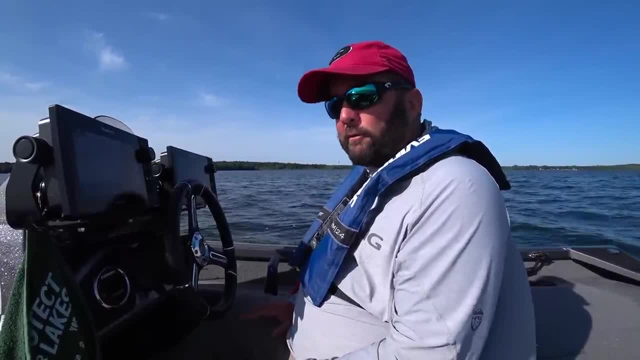 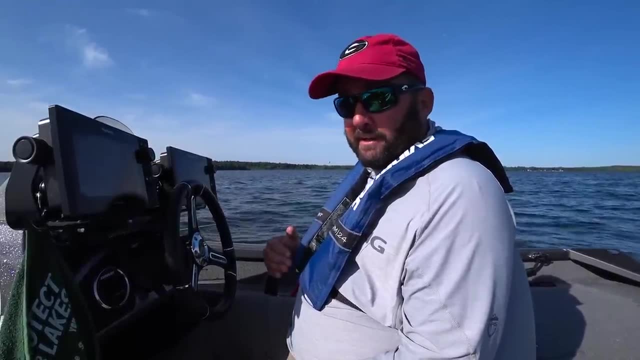 Don't be in a hurry to get back in. The rougher it is, the harder it is to get back in, And I'm going to show you some of the tricks that I've learned through my own experiences- Some really, really scary ones. 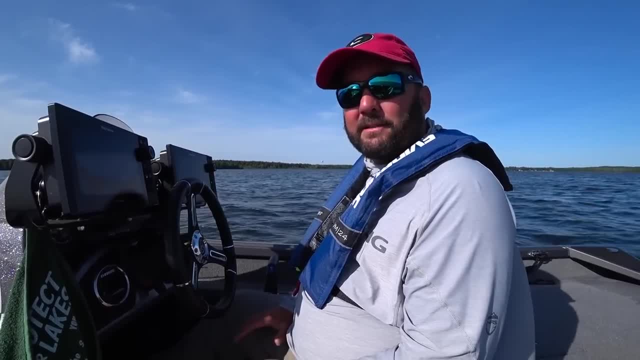 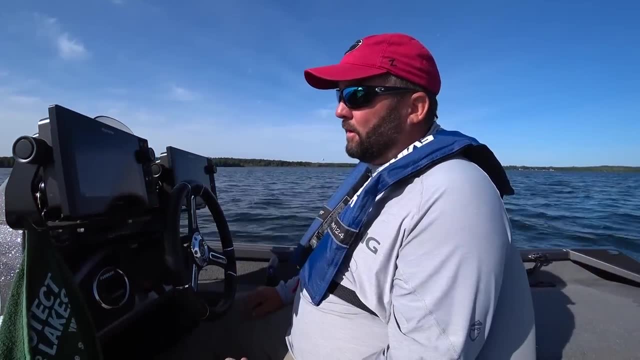 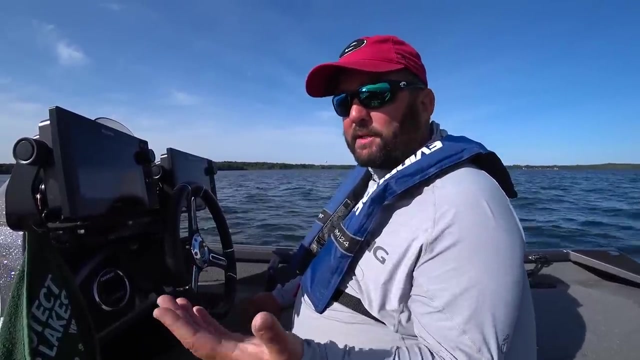 But I've learned how to get myself back to the truck and back to home safely. So when I start to see white caps On the water, I know it's going to be a little bumpy And so. but when I start to see white caps in this boat, 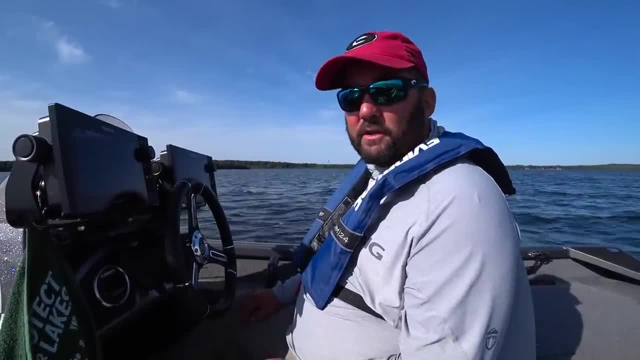 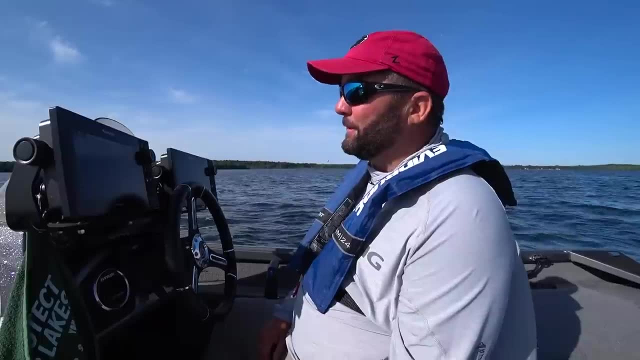 Now, other boats are a little bit different. My Triton was a lot different. If I started seeing white caps, I knew it was going to hurt Going home. I mean, it's one of the old Tritons, It's not one of the new ones. 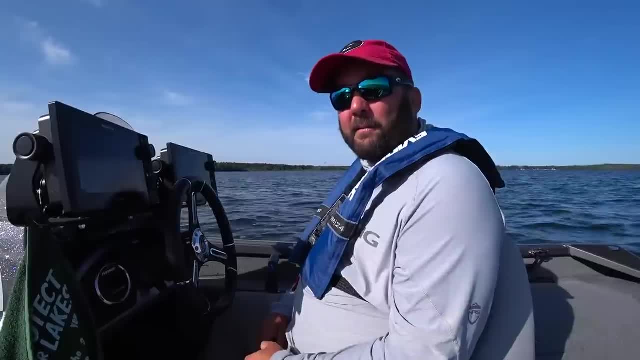 I don't know how they build the new ones, But the old Tritons it flexed so much that it hurt And I knew it was going to be a rough ride back, So I took my time, But I've been in some pretty crazy things. 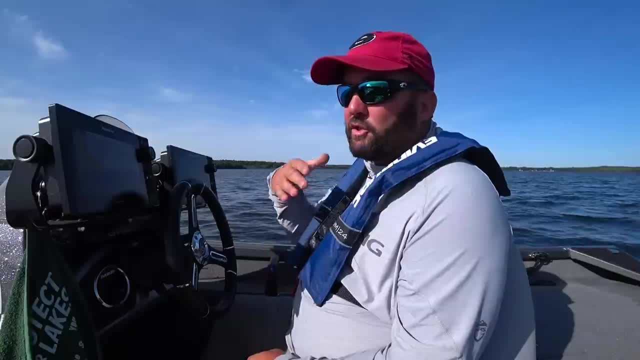 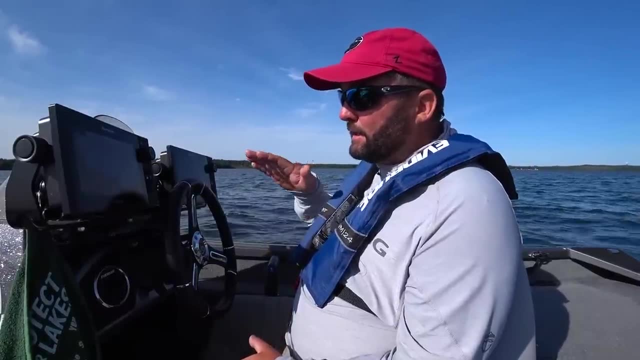 From 4 mile an hour wind to 25 mile an hour wind, And I had to get back, And so what I do is I get the boat going real slow And I trim up. I'm talking these are 3 and 4 foot waves. 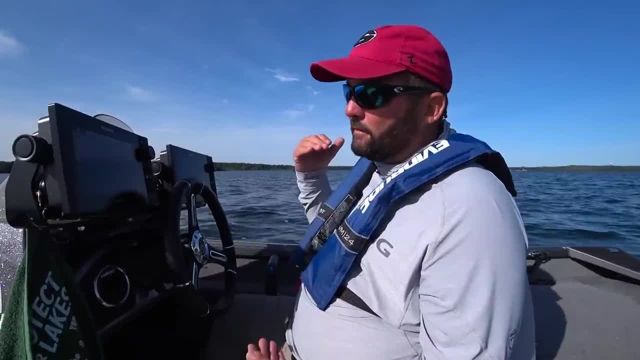 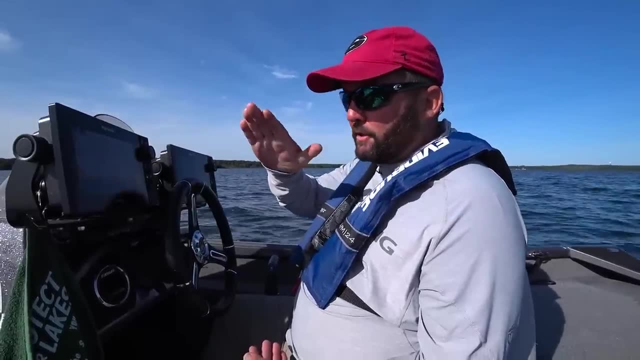 When it's really, really you cannot get up on plane without it being completely and totally dangerous. But I will get the boat going. I will trim up until I've got the front end a little bit in the air And out of the water. 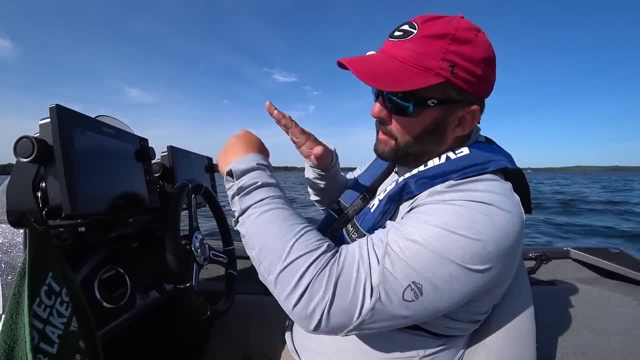 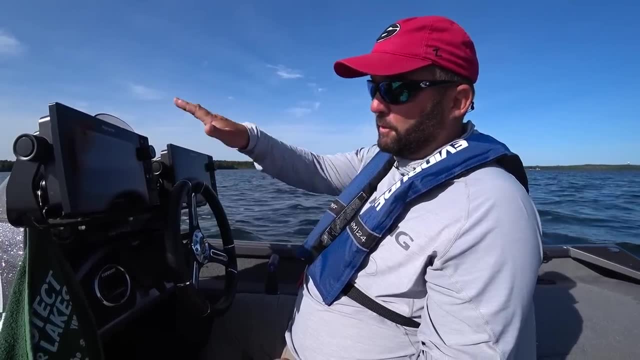 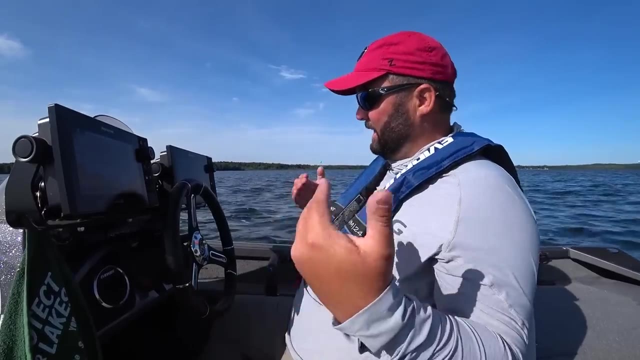 And I want the waves to hit right up in the front third of the boat. I want the waves to hit right there And I, just as long as I'm moving forward, I'm fine, I just keep plowing through- And what that does is it allows the front of that boat to take the brunt of the force of the waves. 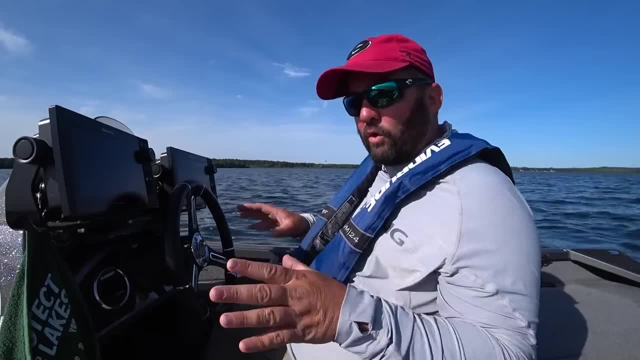 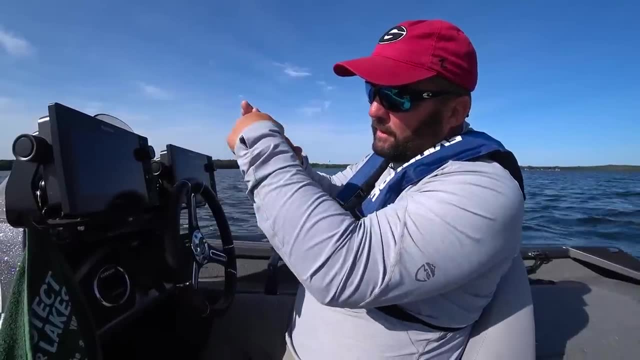 And it keeps you dry And it keeps you moving forward. Now that's the worst case scenario: to get back. Trim up, Get your front end up out of the water and let those waves hit, And you should be able to get back. 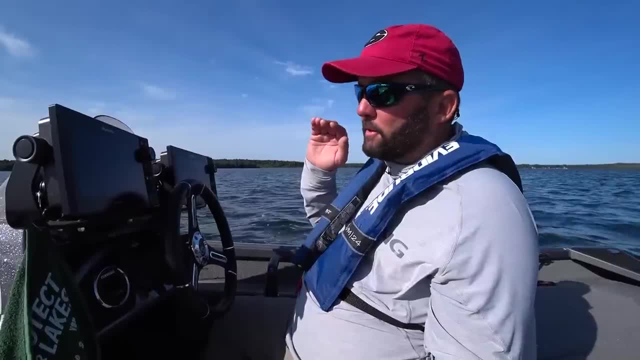 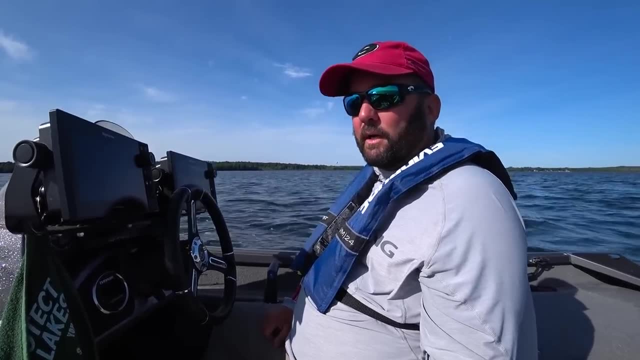 I had one time on Kentucky Lake where it almost seemed like I was going backwards more than I was going forward, And it took me an hour and a half to go 4 miles. And so it can be bad, But you just got to be safe. 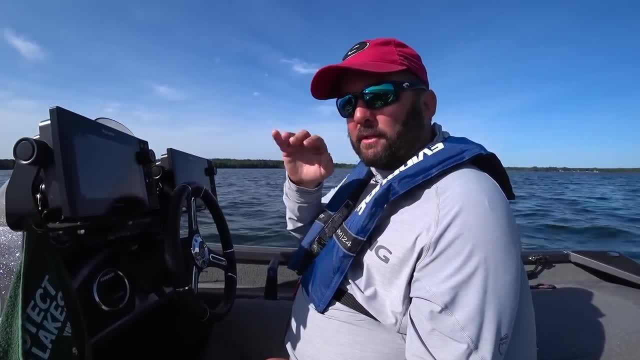 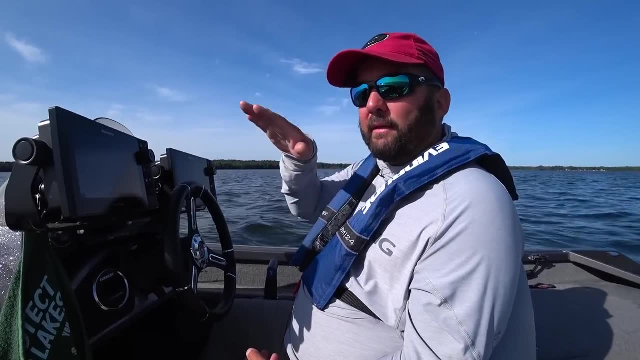 Alright. so now, when you start to see a little bit of white caps and a little bit of chop on the water, There's a couple of things you can do. There's a point in time where they start to get the waves- especially on big lakes like this, they'll start to get rolly. 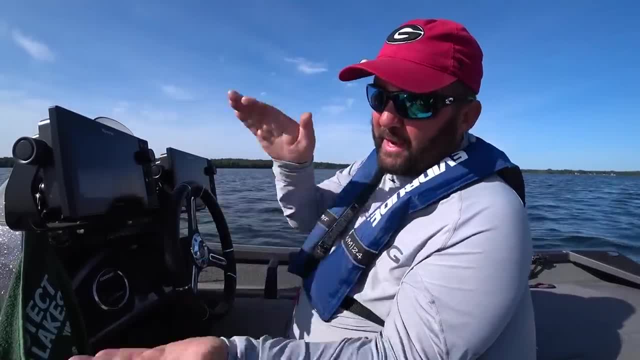 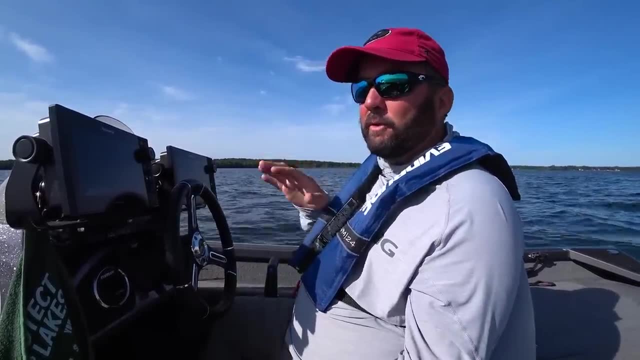 And it really. you'll find that your boat slams into those waves a lot And you don't want to break things. That's when things fall apart, is when you start slamming that boat down, And what I typically will do is just go as fast as I possibly can. 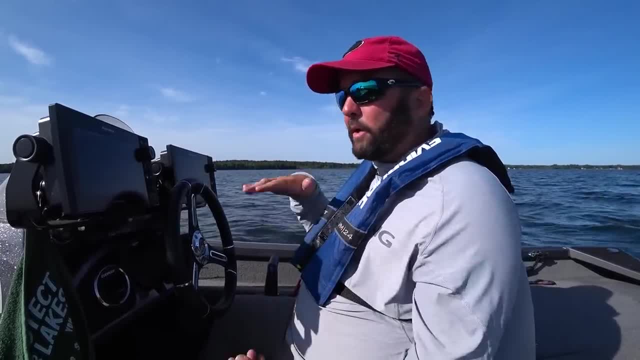 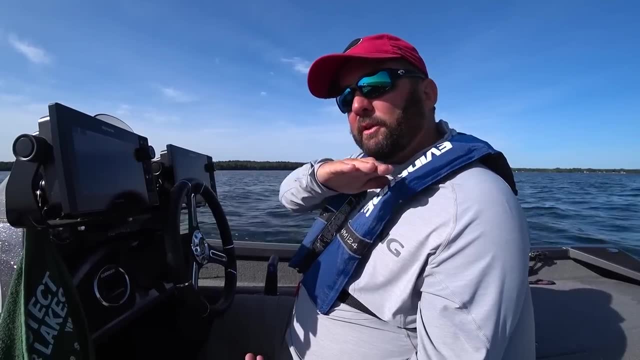 I don't make being up on plane a priority. I just kind of ride them and try to time them and get that speed where it's. you know it's pretty decent, But usually when they're just starting to see white caps you can get up on plane and you can actually skip and ride across a lot of those waves. 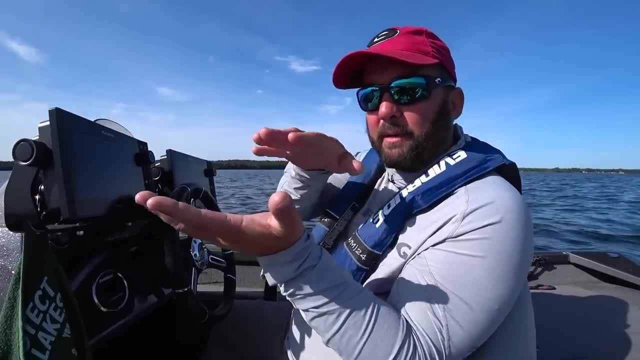 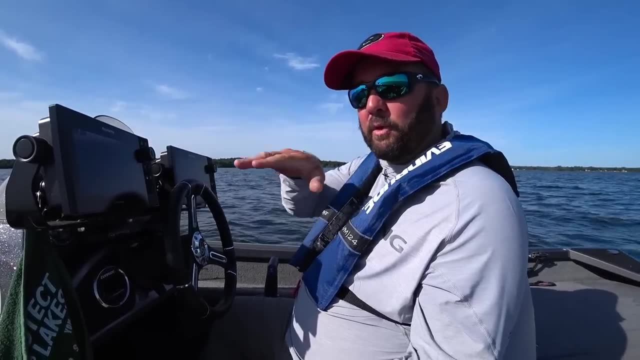 And it'll be just fine. A little bumpy, but not too bad. Fiberglass boats: they can hit those things really good. You can get up on top and just go. They're heavier, so they plow through larger waves a little bit better. 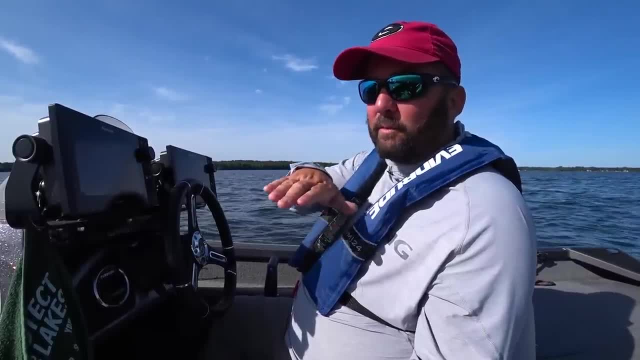 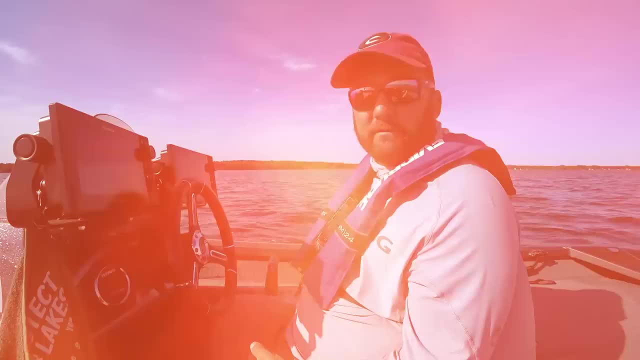 And so, even after, even when the water gets too rough for this one to go full speed on plane, a fiberglass boat can do it, And that's the advantage, One of the advantages, to having a fiberglass, Alright, so more about safety and things. 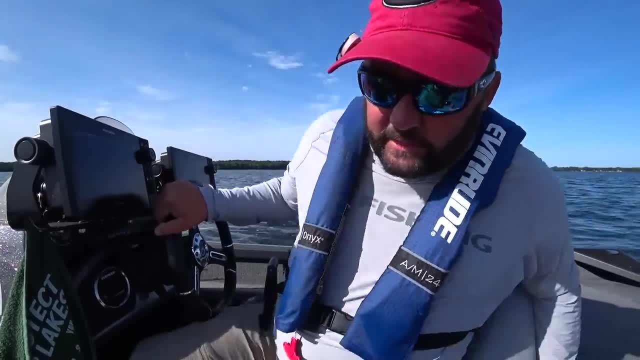 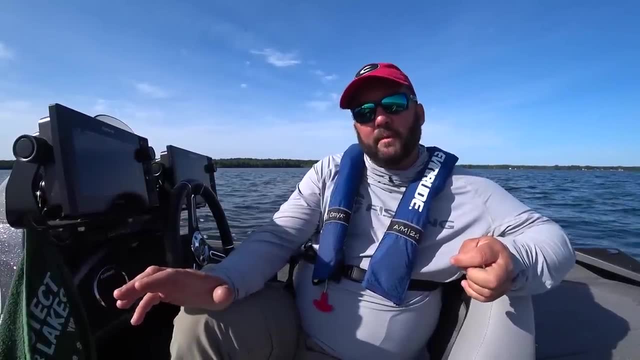 To have in your boat. Now the best thing to do- and I haven't completely finished the rigging of this boat for this- The best thing to do is go to the US Coast Guard website and see what needs to be in the boat. 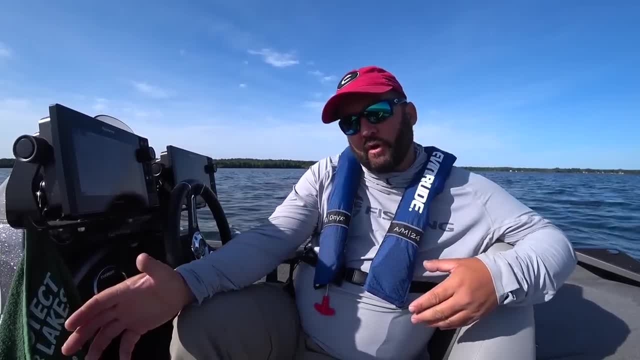 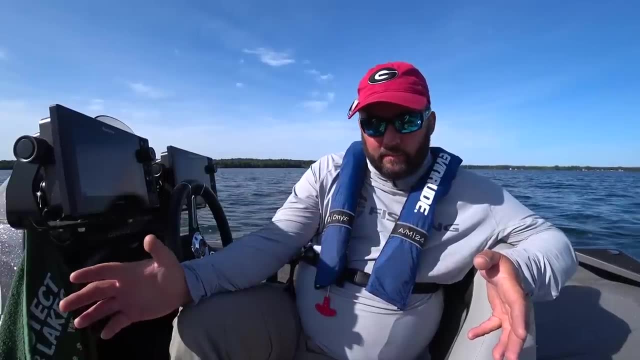 And then pick and choose. Most of what the Coast Guard recommends is for deep, you know, salt water and professional boats and that kind of stuff. But check and see what all you need to have in your boat. It's really cool to get the Coast Guard to check your boat. 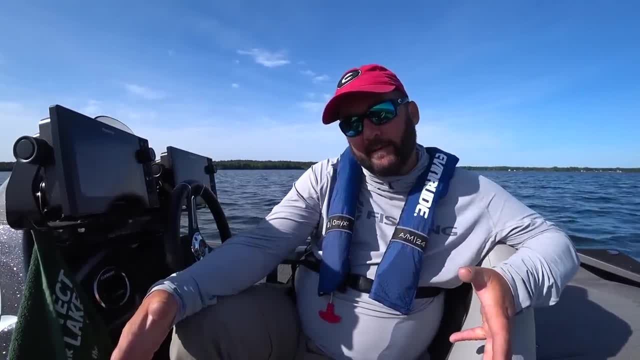 It's really cool to get the Coast Guard to check your boat And you have everything that they have on their list And they'll give you this cool sticker that goes on your boat saying that you've been checked by the Coast Guard. But flares are a good thing. 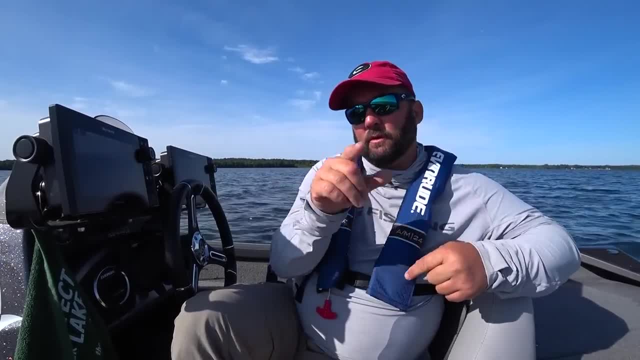 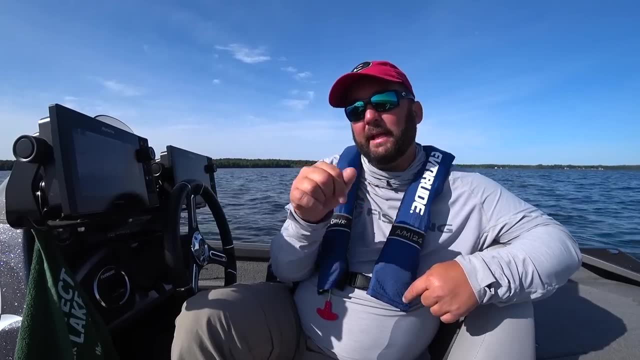 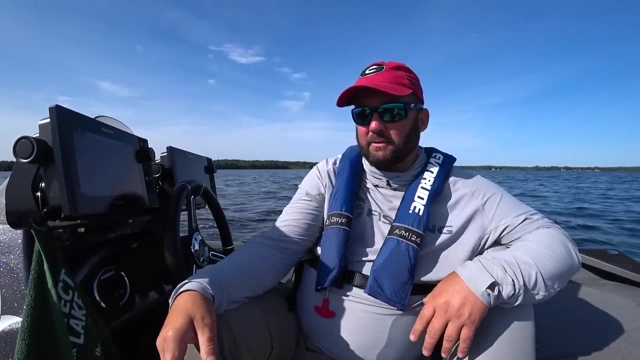 The basics for most of you. Well, let's do this real quick. You can go to your state website and check to see what safety gear they require on your boat. Make sure you have that, And then go to the Coast Guard and get a few of the extra things, just to see. 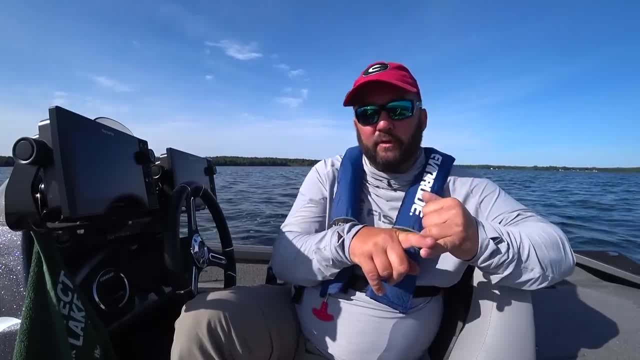 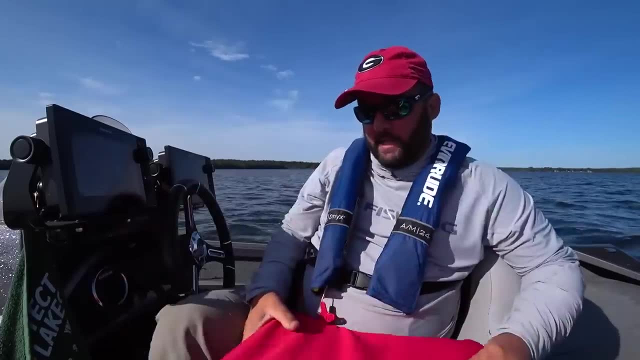 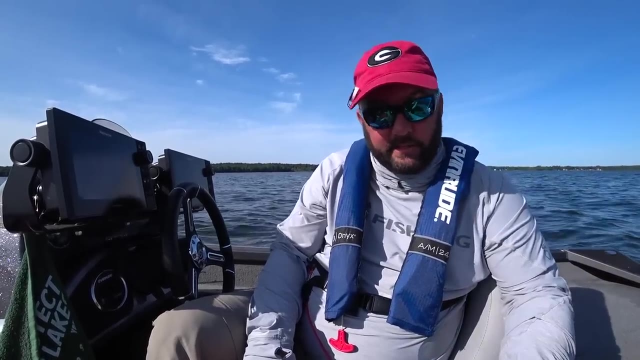 But anyway, usually states require some type of a throw question And mine is up underneath my seat And it has to be easily accessible, So that's a throw question. They also require a. if you have a combustion engine, they require a fire extinguisher, which I have one right up underneath the camera, but I don't want to move it. 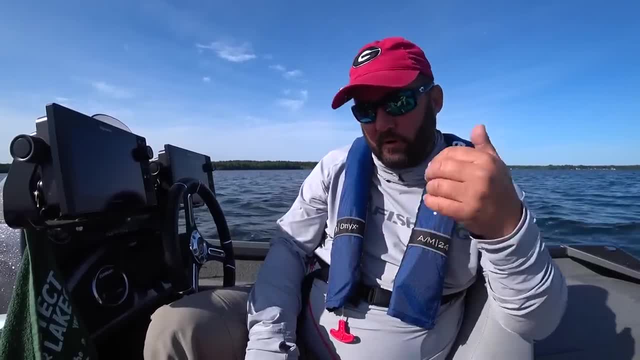 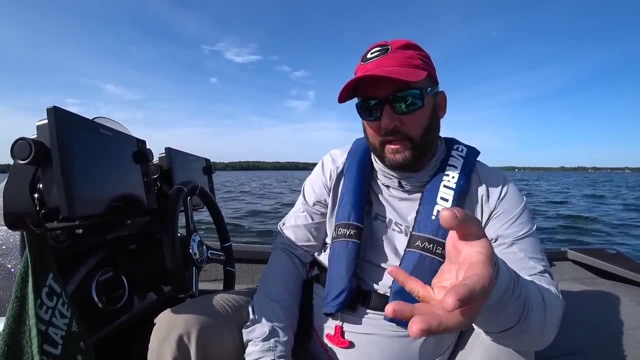 Fire extinguisher, a kill switch that works, PFDs for every person. But just check your list on your state and make sure that you have everything. But the best thing to do is read your state regulations, Read the requirements for your boat and the limitations to your boat. 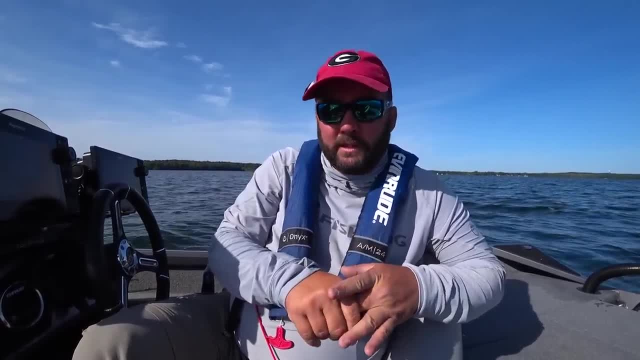 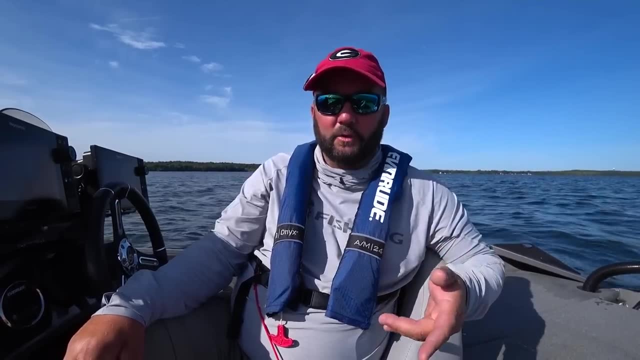 And then go on the Coast Guard website and check and see what they require on a boat And get as much of that as you can. If you're just going to stand in the lakes and stuff like this, it's no big deal. You don't really need the Coast Guard stuff. 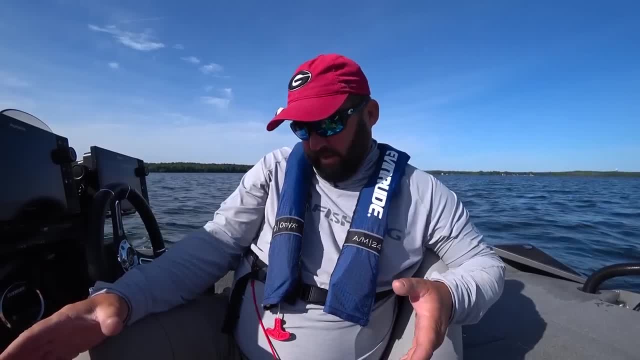 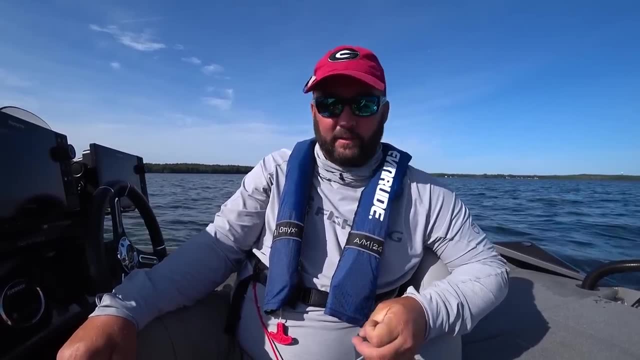 They're just some nice to have And in the next month or two I'm going to have all the stuff that I need for Coast Guard-wise, like flares and things like that. I'm just on too many lakes by myself to not have some way to get help if my cell phone doesn't work and stuff like that. 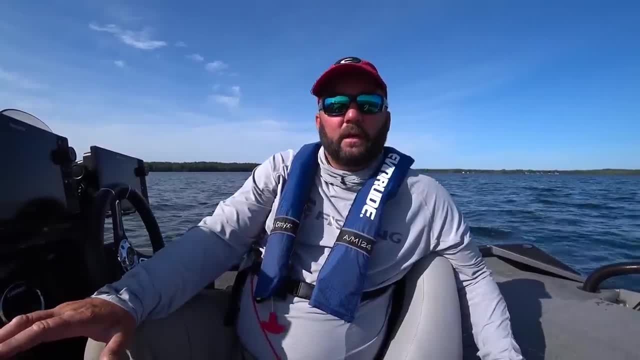 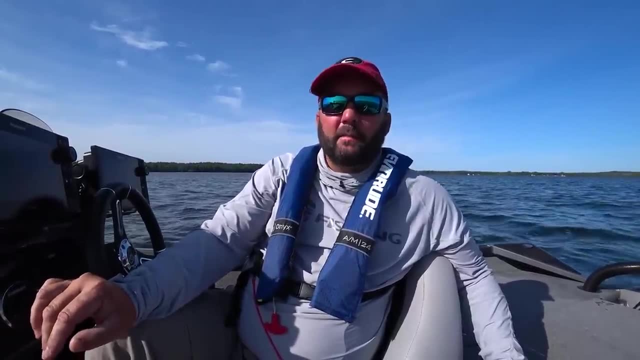 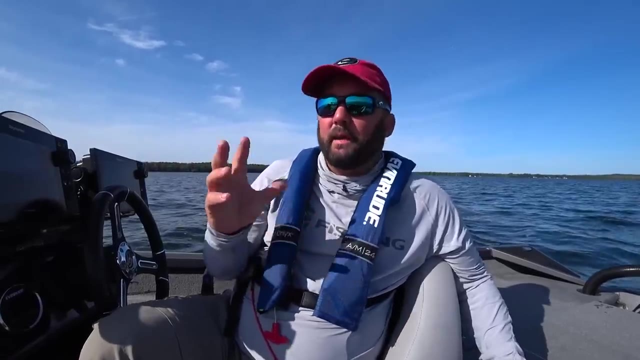 Alright, so now let's talk about on-the-water operation, And this is kind of the part that really bugs me the most. There's a lot of people that don't understand what to do when you're approaching other boats And who has the right-of-way and what side to pass on, and stuff like that. 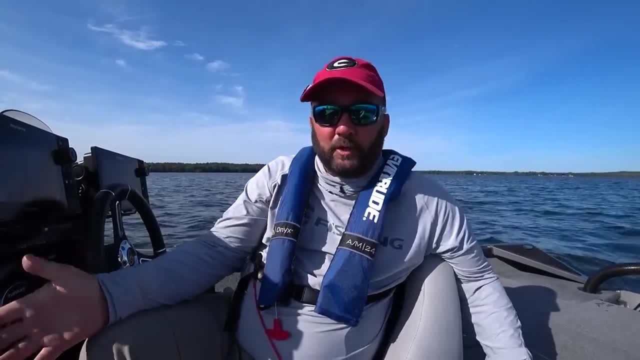 So if you've got a boat coming straight at you- and this is what sucks is, most people don't know this, And so you have to assume they're going to do the wrong thing, But you're supposed to stay to the right of a boat that's approaching you. 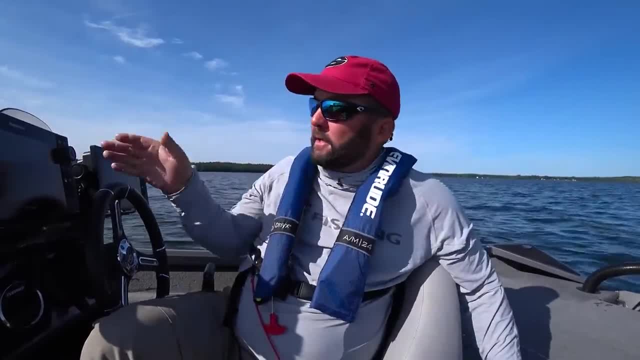 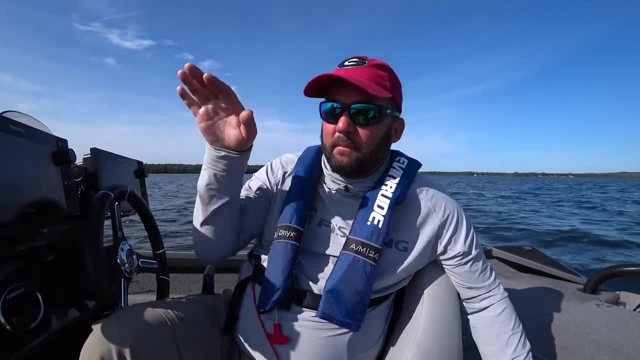 So you pass just like you would on a road, You stay to the right, and they stay to the right, and so on and so forth. And it doesn't always happen that way. If you see somebody sitting down fishing, steer way clear of them. 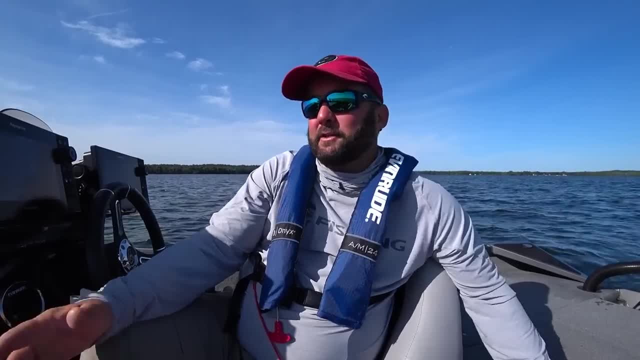 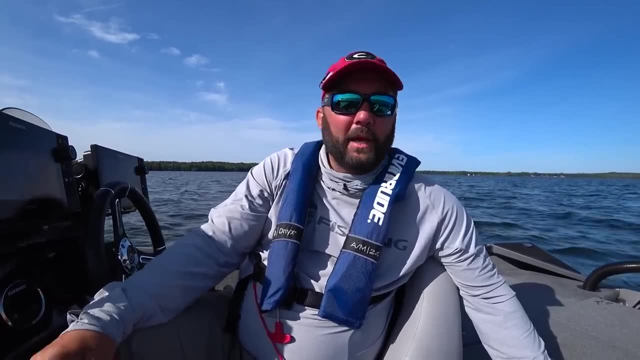 I had a giant boat, about a $200,000 boat, And I'm fishing in two and a half, three foot of water the other day down in Minneapolis And I had this old man just toting along in his $200,000 giant cabin cruiser. 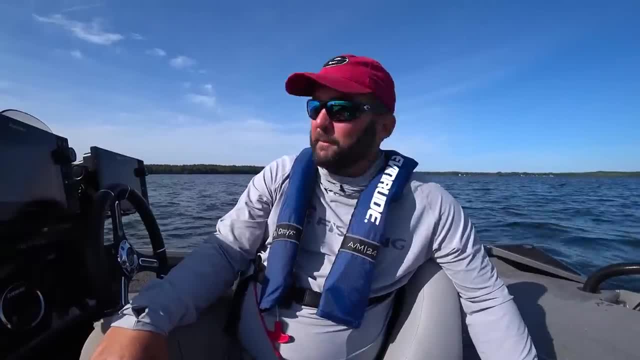 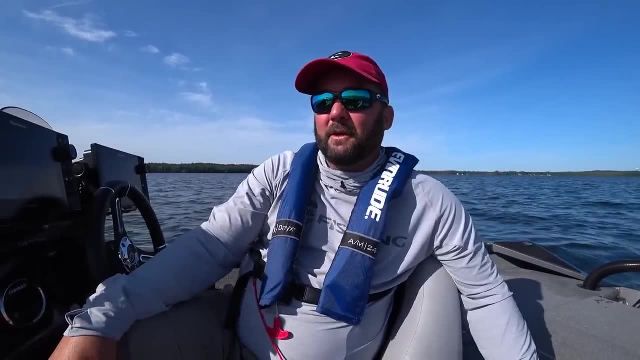 In three foot of water kicking up mud, Had no clue what he was doing And I wanted to scream And he was like right behind me And a lot of people just don't know, They get on a boat and they go And a lot of states don't require boat safety classes or anything. 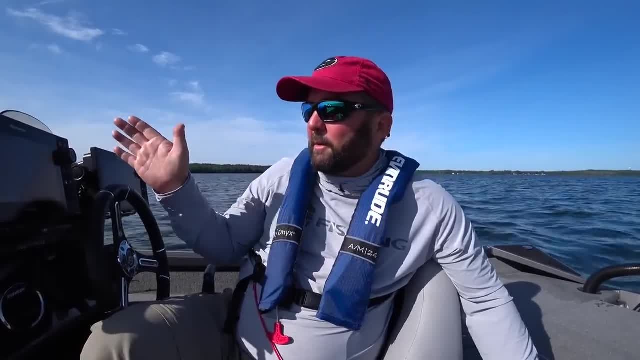 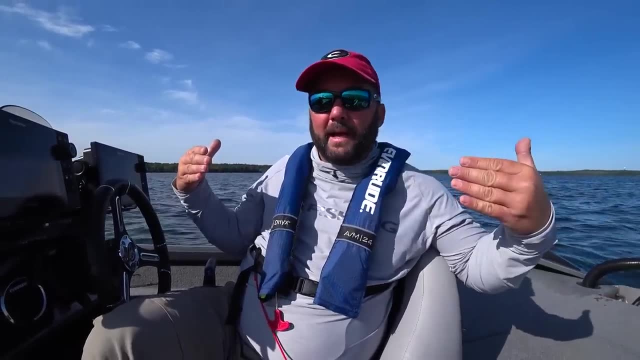 And that's where you get really scary. But know, when you approach a boat you approach them to the right. If you're down in Florida and you're in those really narrow grass lanes And you come around a corner and another boat's coming back at you, 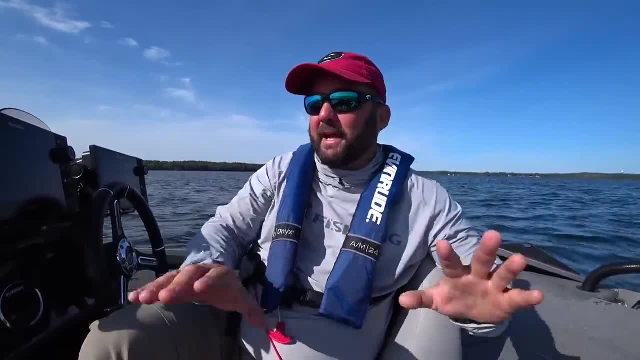 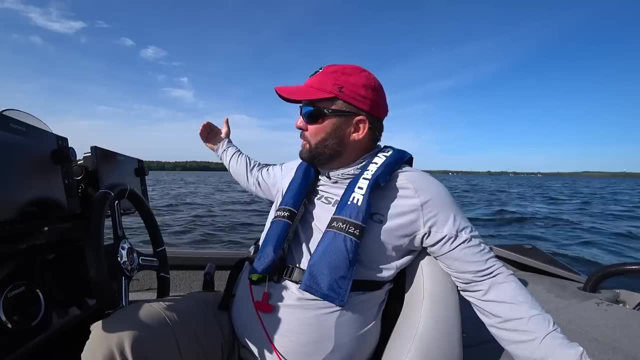 And you're about to get head on. Both of you cut to the right And you put yourself in the grass And nobody gets killed. It's just that kind of stuff Always know you want to stay to the right If you've got a boat approaching this way. 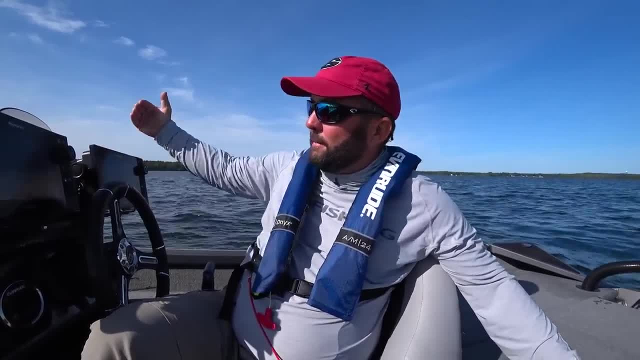 If you're in the navigational channel, you have the right of way, But if you have a boat coming in at 90 degrees And it's best just to give them the right of way, if you can Be courteous on the water-